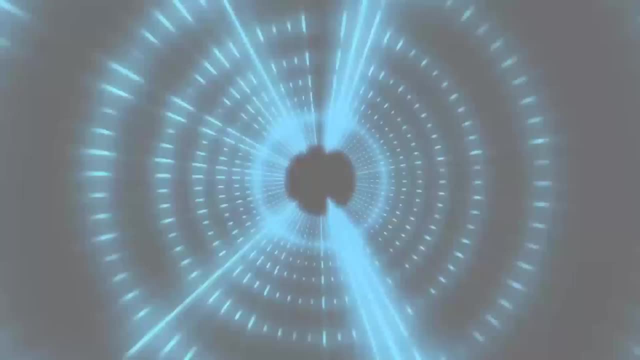 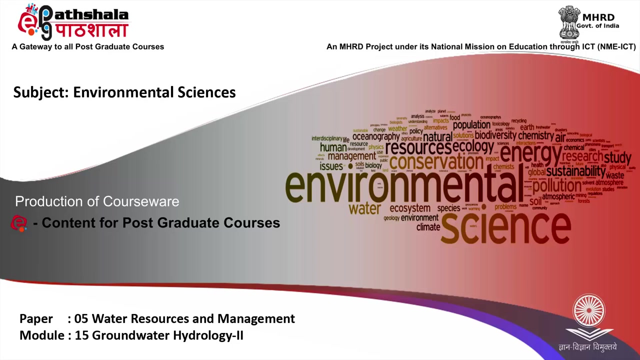 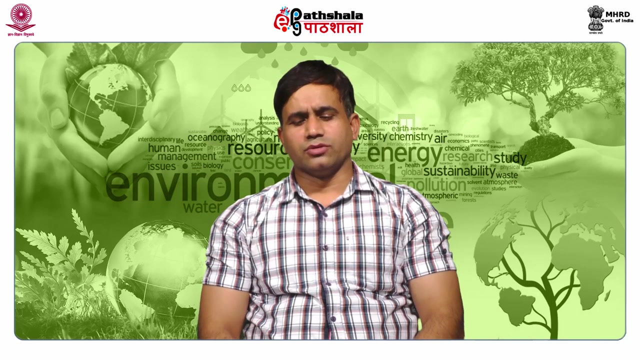 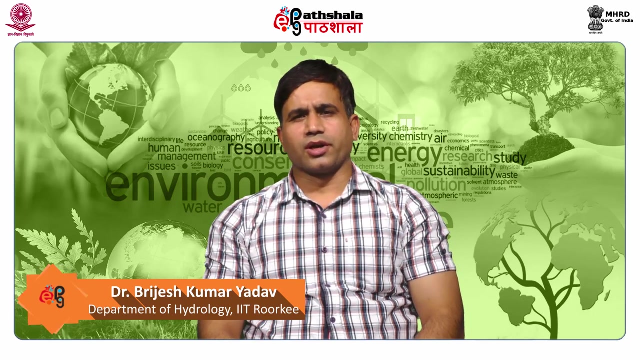 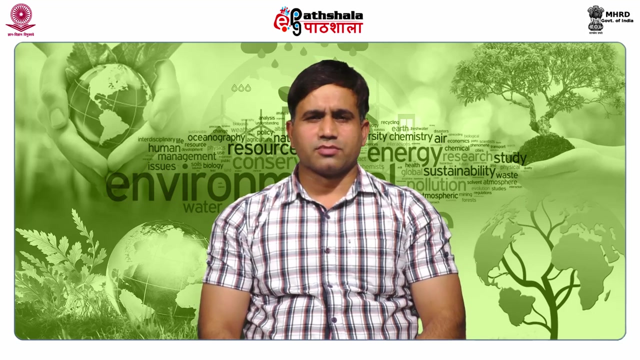 Hello everyone, welcome to this EPG parts allah. In this module we are going to talk about groundwater hydrology. This module is going to discuss about the things which are related to the subsurface water. First, we will introduce the groundwater resources. 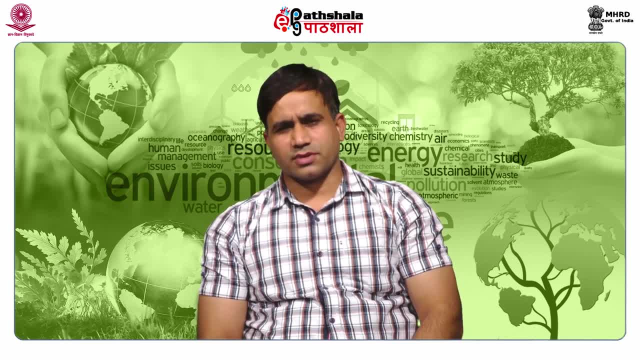 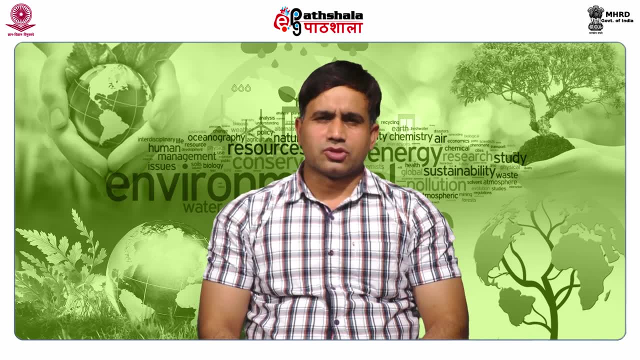 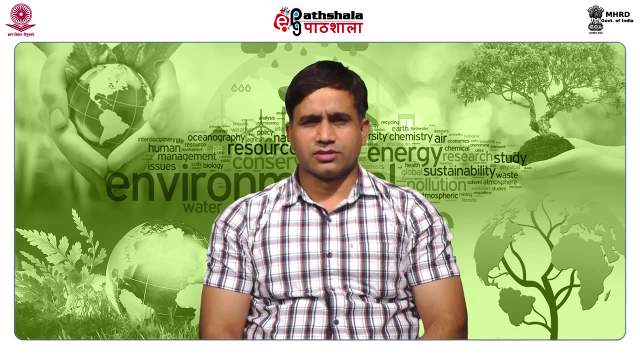 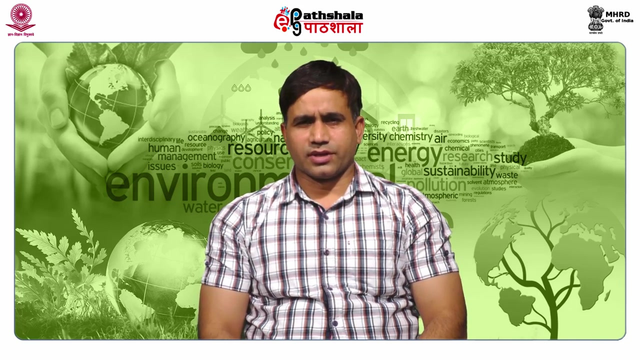 how the groundwater appearance below the subsurface, how it get differentiate from the surface water resources and its importance. We will also talk about the storage of the groundwater by discussing different storage formations like aquifers, their classifications and their characterizations. So what are the different parameters which are going to be used for? 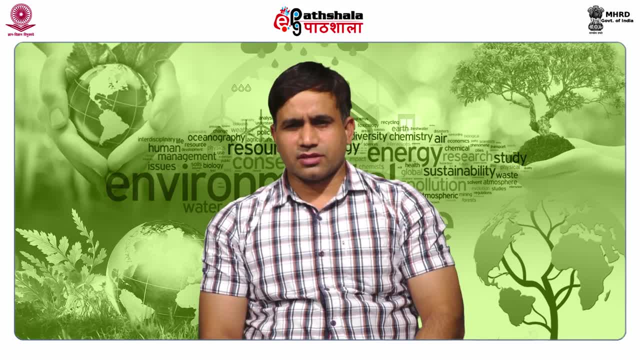 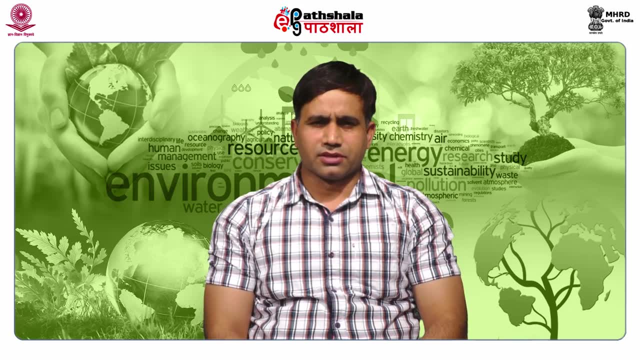 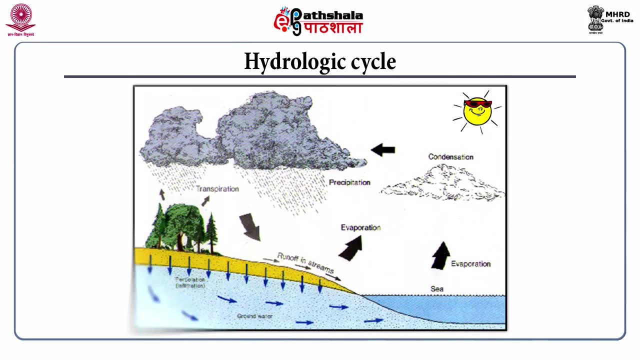 analyzing the groundwater sources are going to be discussed In. last, we will discuss about the different types of the groundwater equations governing equations for the flow and transportation of the pollutants. Here this slide shows the hydrologic cycle. ah, We know that in hydrologic cycle this: 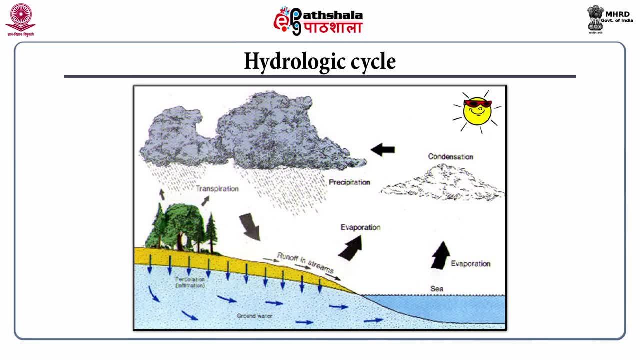 because it is a cycle, So we can take any convenient point for starting Here. I am taking the ocean as the starting point. So ocean water evaporates because of the solar power energy, because solar is the system, is the main source of the energy And because 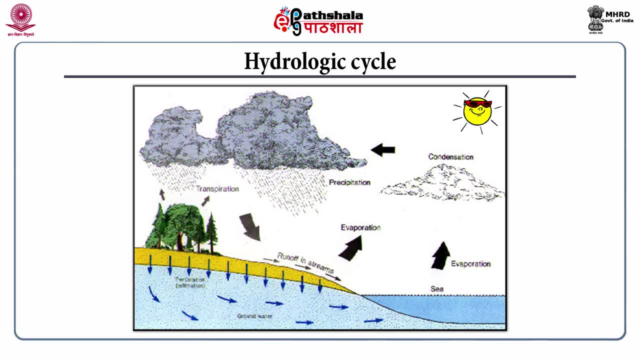 of this radiation, the water starts evaporating from the sea, It goes into the above the surface, above lying atmosphere, ah, making clouds. because of the condensation and because of this global circulation, these clouds moves towards the landmass. After reaching to the landmass, 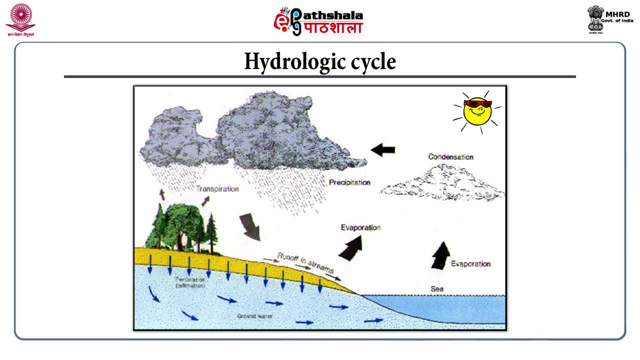 ah, favorable conditions are received and the precipitations start taking place. So from the atmosphere, the precipitations comes from the to the ground. after reaching to this rainfall to the ground surface. PAR inconsistency as Wei Zan Guai, previous slideishment fromittion 24.46, q.11, q.14 q. transcendence. 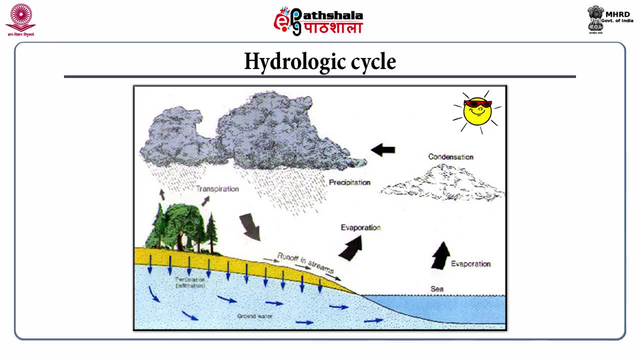 to Egir: q.23, 15.18, q.23, 15.39, q.33, 15.32, q.23, 15.42, 15. stimulateực portion of this precipitation start running over the surface, which is known as surface runoff. 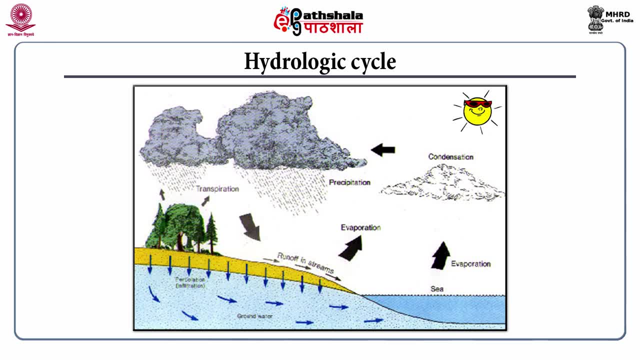 Some goes back into the atmosphere in form of the evaporation or the transpiration loss, and the remaining amount goes into the subsurface which is shown by the vertical arrows in this figure. So this is known as the infiltration. So in surface water hydrology we consider: 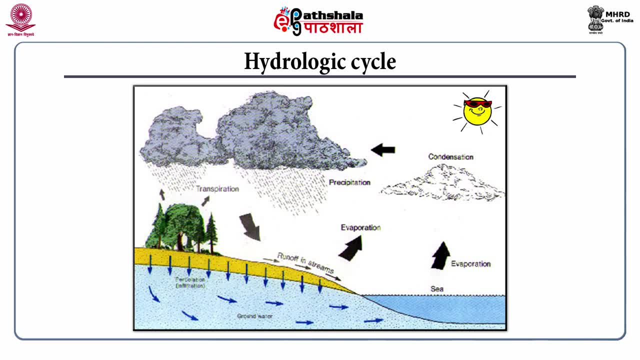 infiltration as a losses abstraction, because it is not contributing to the surface water sources. However, in groundwater hydrology, this is the main influx which is going to rejuvenate the groundwater sources. So that is going to the main source for recharging our underlying groundwater aquifers. Now, once this infiltrated water reaching to the water table, 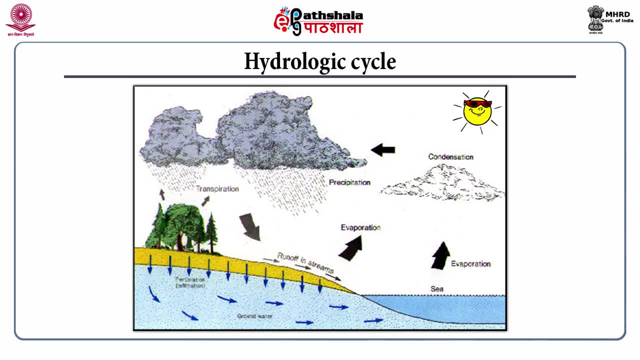 it is started moving mostly in horizontal or lateral directions and ultimately meeting to the surrounding water bodies, which completes this entire hydrologic cycle. So the focus of this module is going to be on this movement of this subsurface water below the ground surface, particularly in saturated zone, which is denoted by light blue area here. 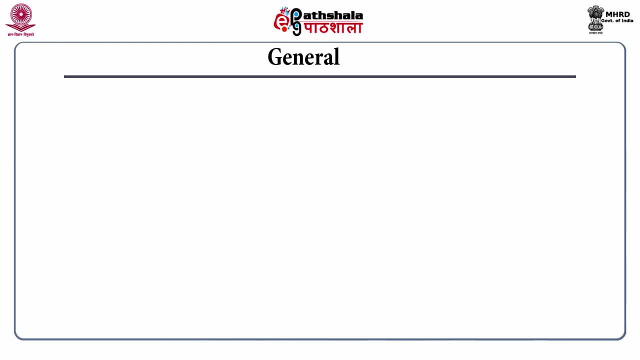 Now the topic of this module is groundwater hydrology. So we know the hydrology is a science of water and this deals with the occurrence, its circulation and distribution over the planet earth and in its surrounding atmosphere. When somebody says groundwater hydrology, or hydrogeology or geohydrology, So hydrogeology, it encompasses the interrelationship of 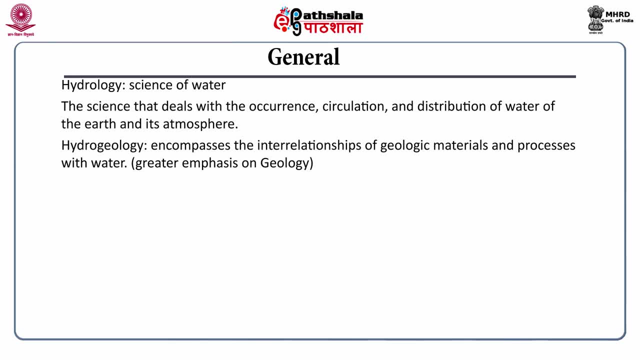 geological material and processes with water, and geohydrology, mostly used as a synonym for the hydrogeology, though it is more you know- properly describes the engineering field dealing with the subsurface hydrology. So sun is known by father, or father is known by sun. 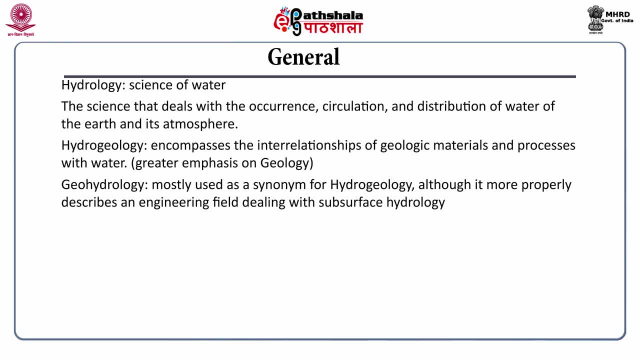 So the main focus of hydrogeology and geohydrology is to understand the interaction of the water with the surrounding geological material. The objective of, you know, understanding groundwater hydrology is going to be threefold. The first one is the groundwater exploration and 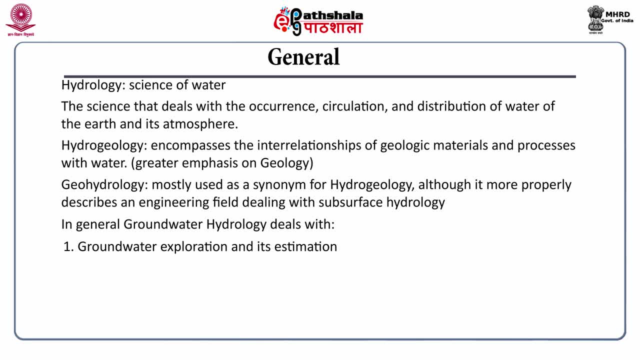 its estimation. So first we will try to explore whether the groundwater is available or not, and if it is available, then what is the total quantity? how can we estimate the groundwater? The second objective is to study of the groundwater hydraulics. This is the core of this: groundwater hydraulics. 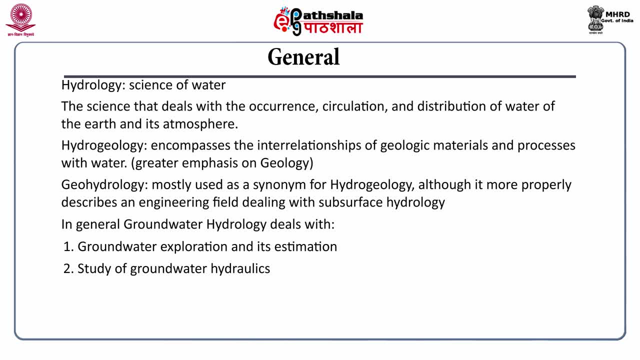 we understand the main mechanisms and the processes which governs the movement of the groundwater below our surface. And the last one, that is not the least, is the study of the groundwater problems and management. Like other natural resources, groundwater resources are also facing many problems. So what are the issues which are pertaining to the groundwater and how can we? 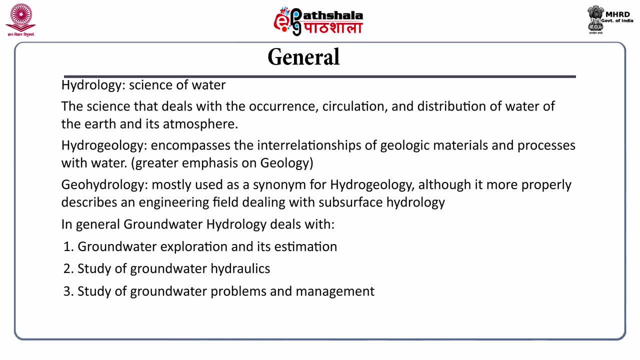 remediate, can manage our groundwater resources or comes under this three objective. number three, Groundwater study, is important for engineering, working, geological studies, water supply development and it plays an important role in petroleum engineering also, where we talk mostly about the multi-phase flow where the hydrocarbon oils do not mix with the water In this picture. 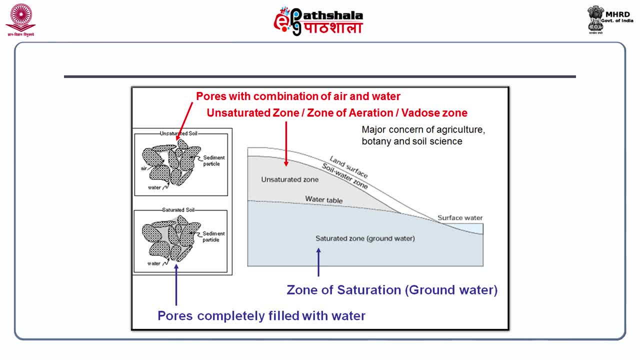 here. this shows the storage of the groundwater. So this is the picture where the entire zone is divided in two part. The top portion, starting from the land surface to the groundwater table, is known as unsaturated water. Unsaturated water: the soil particles are partially filled by air. 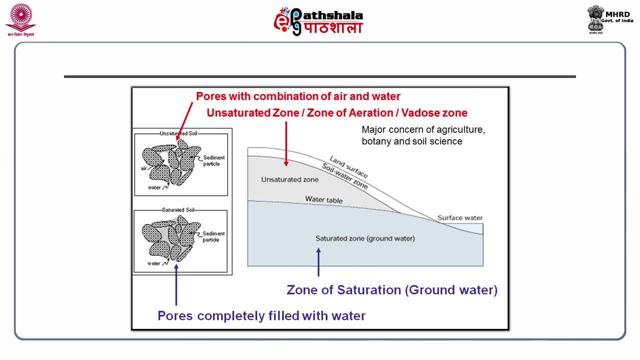 and partially by water. So and the below, the groundwater table, which is known as the groundwater source also, that is, this completely saturated zone where all the openings between the soil particles are completely filled by water, And the water table divides this saturated zone with the. 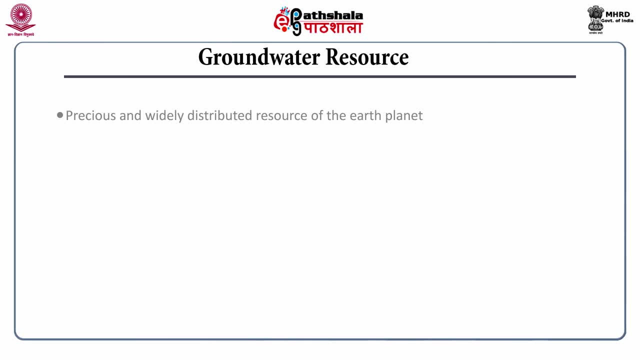 unsaturated zone. Groundwater sources are very precious, like other natural resources, And it is widely distributed resources over this earth planet. Unlike other mineral sources, groundwater gets its annual replenishment from the natural precipitation And groundwater is the largest source of the fresh water on planet earth, excluding the ice caps and glaciers. 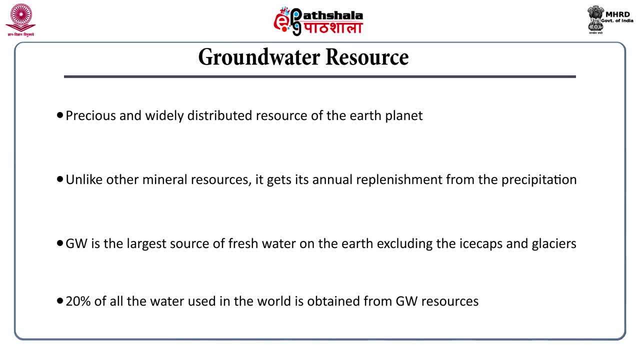 And right now more than 20 percent of all the water use in the world is obtained from groundwater resources, So we have the huge potential for developing our groundwater sources. Now let us compare groundwater with the surface water sources. If you take the extent groundwater, 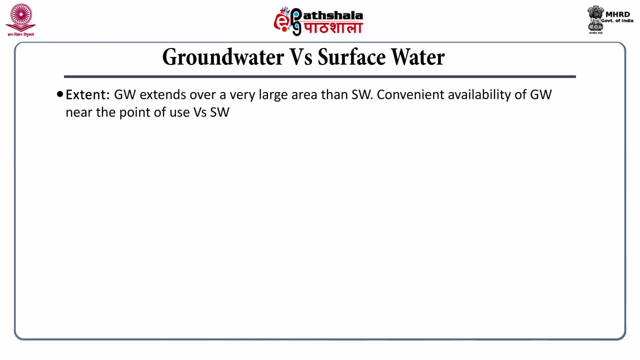 extends over a very large area as compared to the surface water, And that is why the groundwater is explored at a convenient availability at the point of use, as compared to the surface water Availability point of view. exploration of groundwater needs energy. We cannot take out. 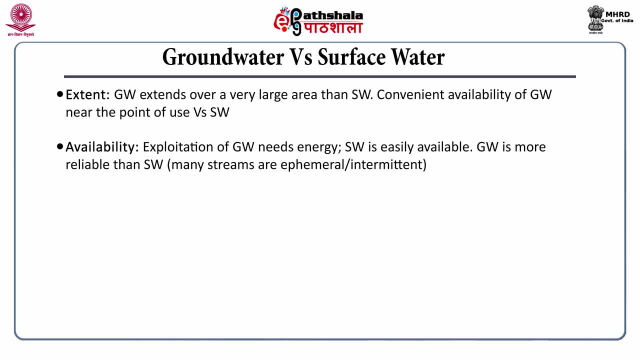 the groundwater at the surface without any pumping, So surface water is easily available and groundwater is more reliable than the surface water. Why groundwater is more reliable? because during these natural disasters, like droughts or the floods, surface water is not fit for drinking or it is not available And the only source, ultimate source, is the groundwater Temperature. 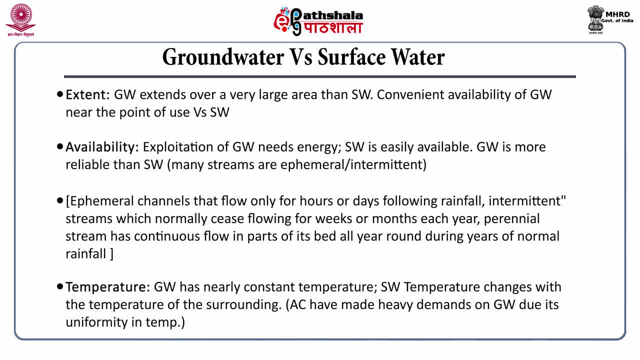 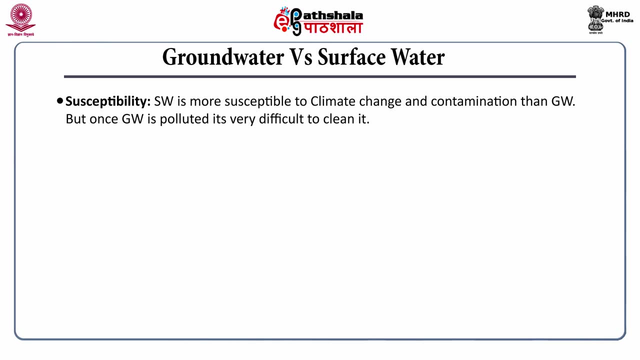 groundwater has nearly constant temperature as compared to the surface water resources And that is the reason that most of the industry they like to extract the groundwater resources for their utilization Susceptibility. Surface water is more susceptible to the climate change as well as for contamination as compared to the groundwater, Because groundwater polluting. 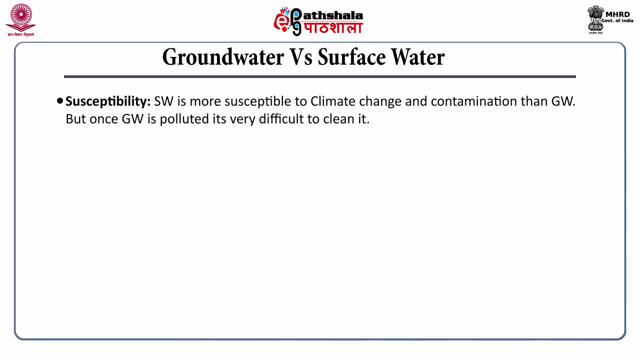 the groundwater is not easy task because it is, you know, covered from the varroous zone, unsaturated zone, Where is lying between the groundwater table and the surface. However, once the groundwater polluted, its decontamination is extremely difficult. This most of project point of view. groundwater projects are usually single. 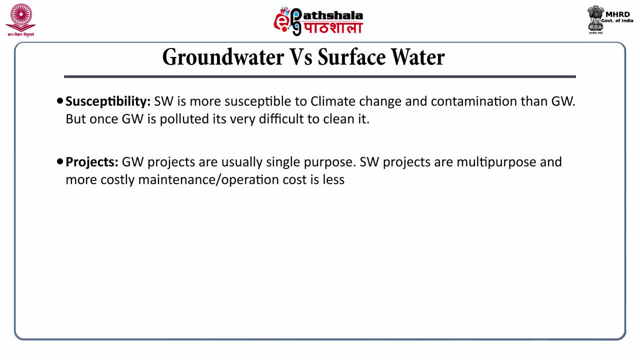 purpose. for example, we develop wells, hydraulic wells, for maybe irrigation point of view or for drinking water point of view or for some other industrial point of view. but surface water projects are in general multi-purpose and more costly in compared to the surface water groundwater maintenance response of the project. it is very difficult to predict the response of an aquifer. 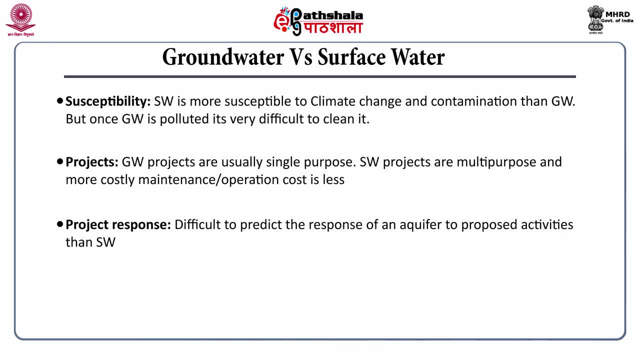 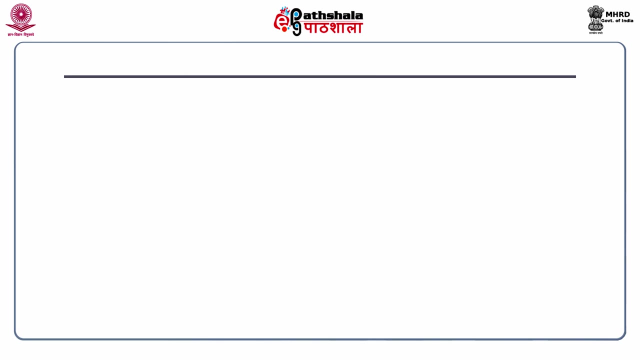 that is the groundwater storage media as proposed to a activity surface activity quality. groundwater quality in general is considered better than the surface water and we consider it is mostly free from the, the pathogens or the virus which are, you know, responsible for many water diseases. now come to that how this groundwater is get stored in. 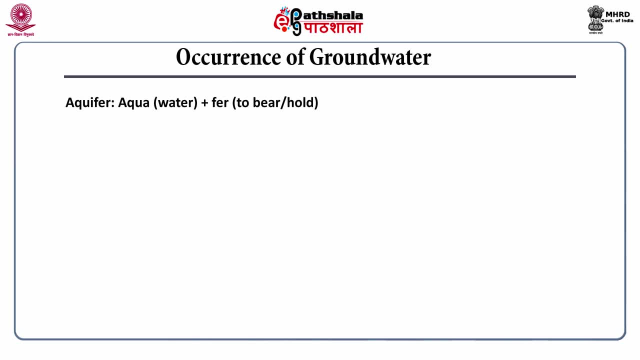 our subsurface. so aquifer is the term which we will use in groundwater for denoting the storage of the, the subsurface water. this aquifer is made of two words: aqua means water plus for to be able to hold, so water bearing geological formations are called as aquifers. there are two important property of aquifer. the first: it must contain. 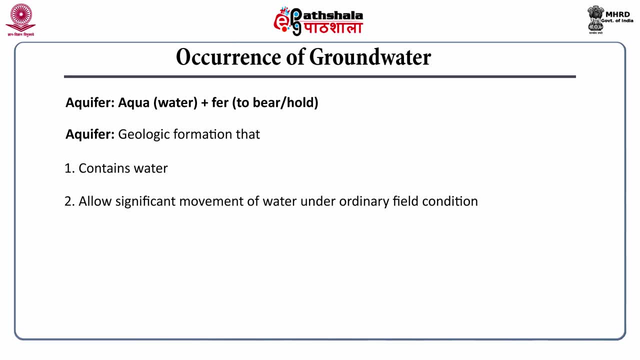 water. the second: it should allow significant movement of water under ordinary field conditions. so any geological material addressing these two properties can be called aquifer. so aquifer must contain the water and it should allow significant movement of the water without any external pressure. so an ability to store and transmit the water is the main property of the aquifer. 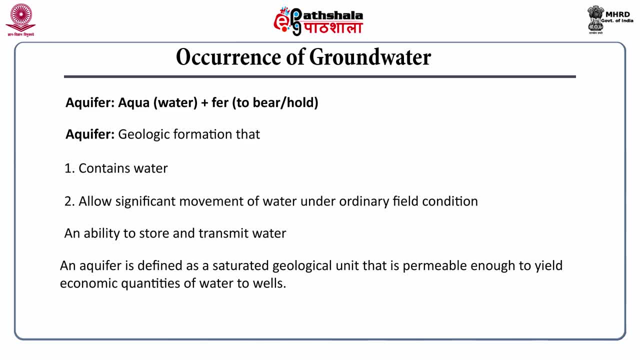 an aquifer. it is defined as the saturated geological unit that is permeable enough to yield economic quantities of water to wells which are drilled into the subsurface to fish throughout, and that is a very important component that we will see in the future aquifer, offering more minerals and balance the inner surface. if you ring for FORMON. 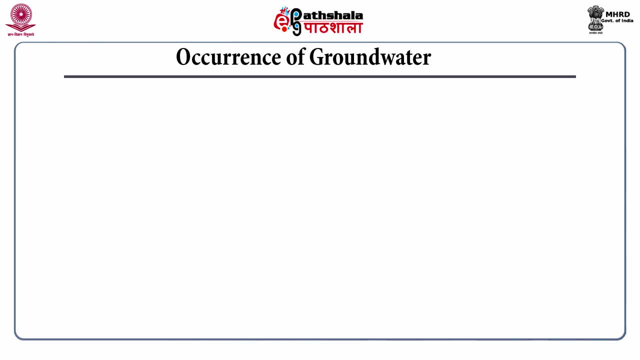 you should be able to mark down Arctur. if you think, where is this Arctur? what to expect? this surface, which we call aquifer, is a water bearing formation. amount of the water, but the movement of the water through this clay formation is going. 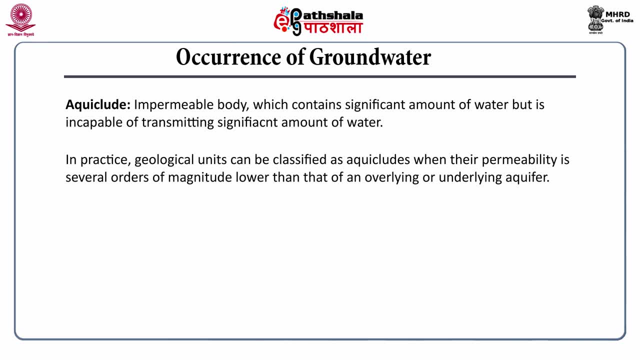 to be very slow, insignificant, So they are called as acuclid, Acutard. these are the geological units of semi impervious nature. They transmits the water at very lower rate as compared to an aquifer, but quite fast as compared to acuclid. So acutard are somewhere. 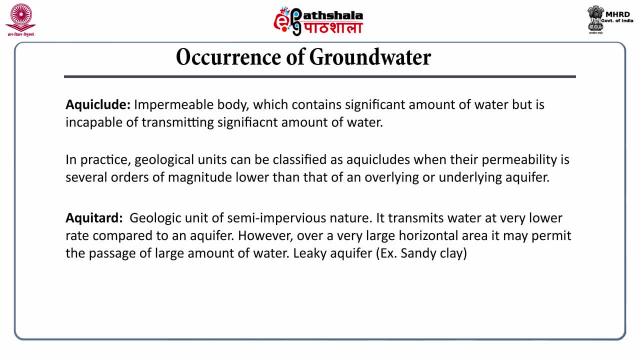 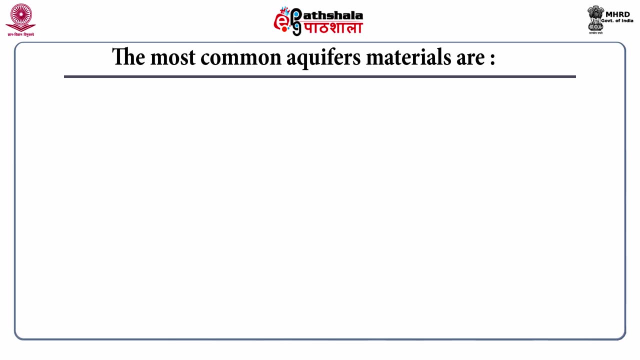 between aquifer and acuclude, And the last one is the aquifuge. Aquifuge neither contains water and nor allows the movement of the water. Any unfractured hard rock or the solid granite is the example of aquifuge. The most common aquifer materials are the unconsolidated sand. 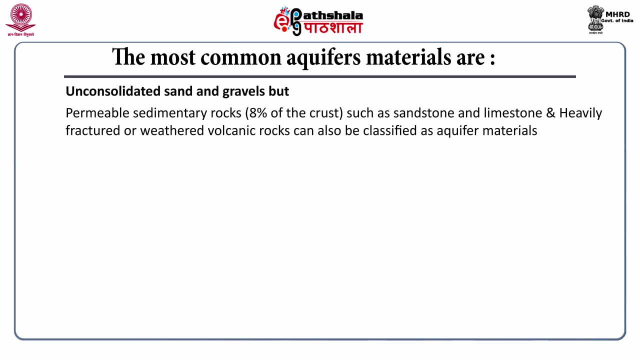 and the gravel mix, but permeable sedimentary rocks, which is making 8 percent of our earth crust, such as this sandy stone, limestone And heavily fractured or the weathered volcanic rocks, can also be classified as a good aquifer materials. And these are the you know, some pictures which showing the sandy stones and 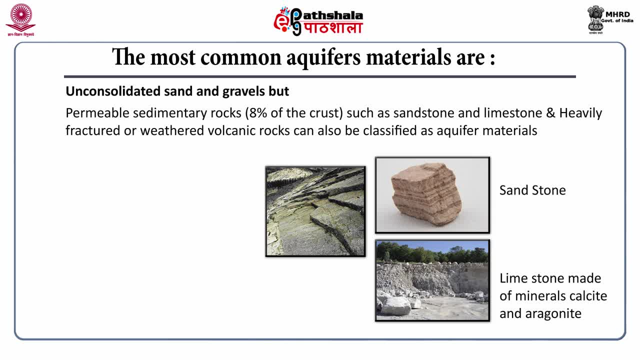 other type of the aquifer media which is going to be comprised store this subsurface water. The main function of the aquifer are 4.. The first one, the source of the water. the second is the storage reservoir. Water gets stored in the aquifers in voids of the geological 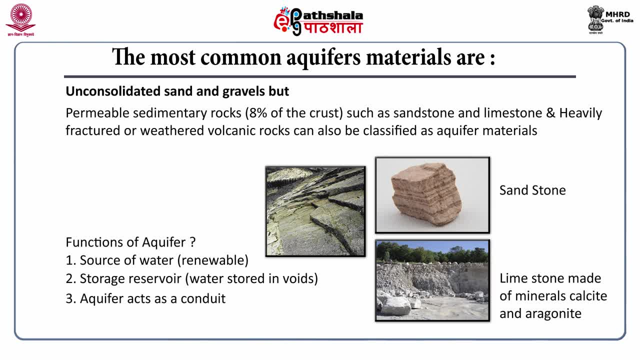 material by which the aquifer is stored made of. The third one is aquifer acts as a conduit. It transmits the water from one place to another place. and the last one is the aquifer acts like a filter plant. that is very important when we talk about the groundwater quality, So when groundwater moves through, 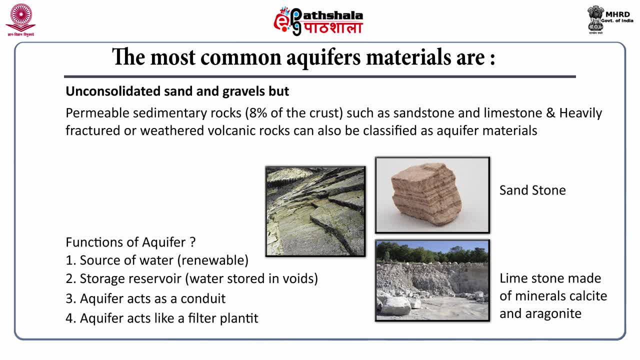 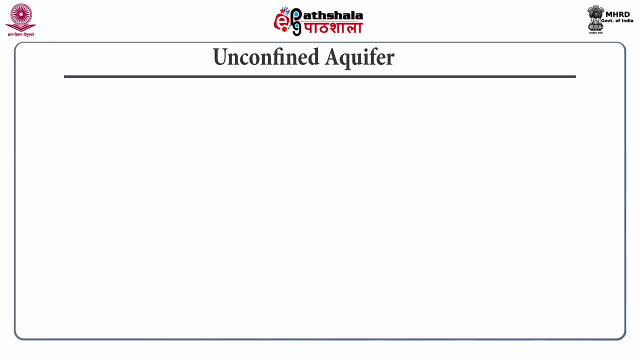 the aquifer. its water quality is gets improved because of this filtration or degradation processes. Now let us classify the different geological formations which contains water known as aquifer. So mainly aquifers are classified as unconfined and confined aquifer. So this slide shows a unconfined aquifer and aquifer. 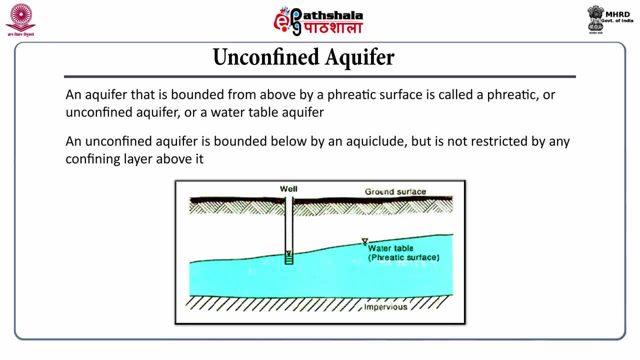 that is bounded from above by a phreatic surface. Phreatic surface means water table, So upper boundary is the groundwater table and the lower boundary is an impervious barrier. It is a clay liner, So water cannot move across this clay liner. So such type of the aquifers- 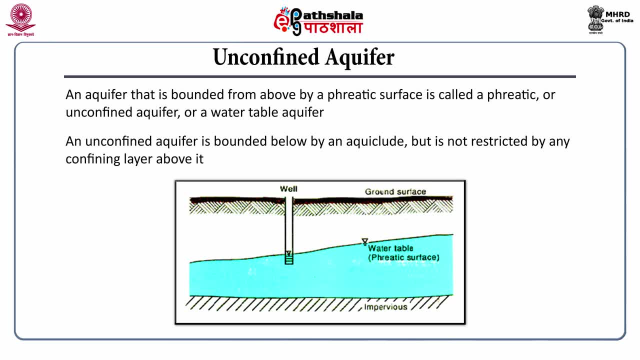 are known as unconfined aquifer. Unconfined aquifer because they are only confined from the bottom layer. The upper layer is the atmospheric pressure representing the groundwater table. So when somebody is going to drill the water in such type of the aquifer material, the water table in well 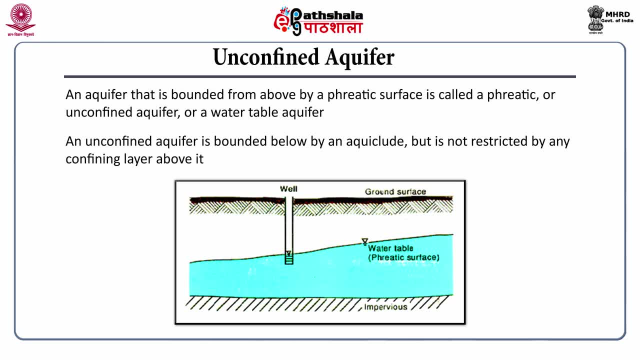 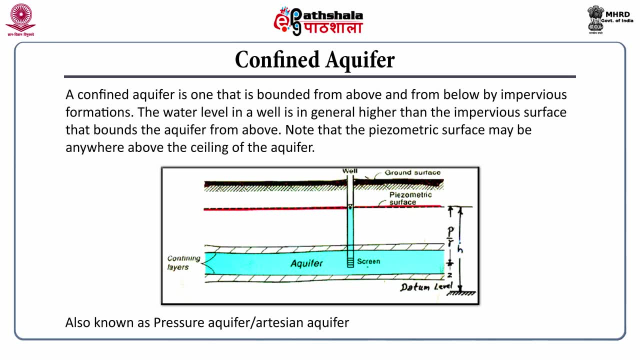 is going to be at similar location as groundwater table Confined aquifer. a confined aquifer is one that is bounded from above and from below by impervious formations, So both the top and the lower boundary are impervious barrier and the water in general. 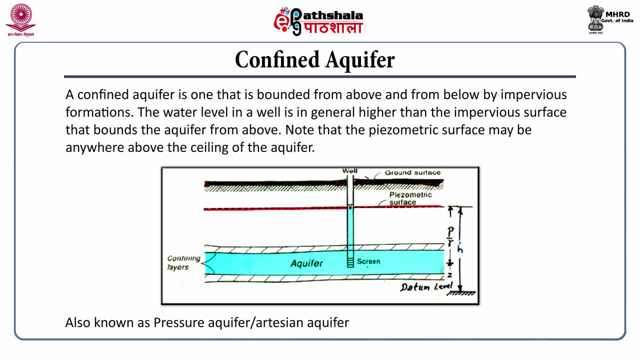 is stored under pressure. So when we drill a well, the water level in such type of the aquifer is going to rise above the upper, you know, boundary of the confined aquifer, and that is known as physiometric surface, which is denoted by this red line here. So the 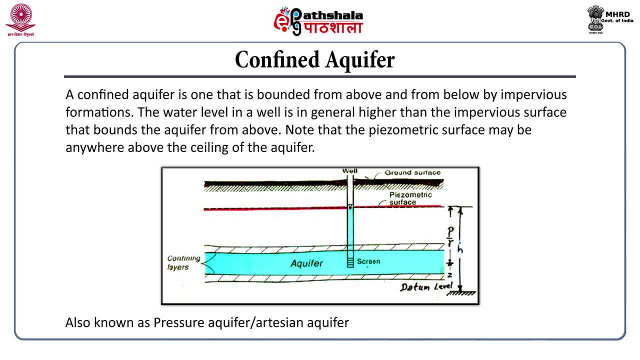 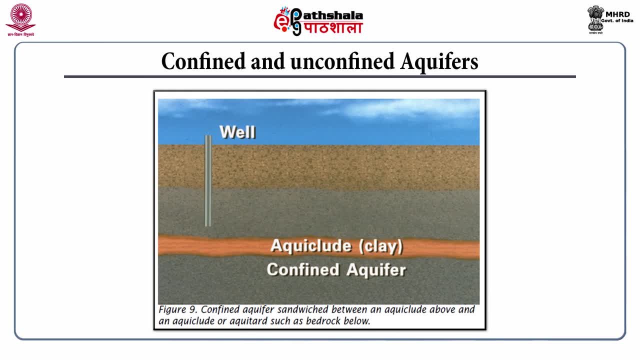 physiometric surface is going to be above to the upper confining layer of the confined aquifer. This is the picture which shows the difference between confined and unconfined aquifer, where a well is drilled here and that starts from the water table to the clay liner that is. 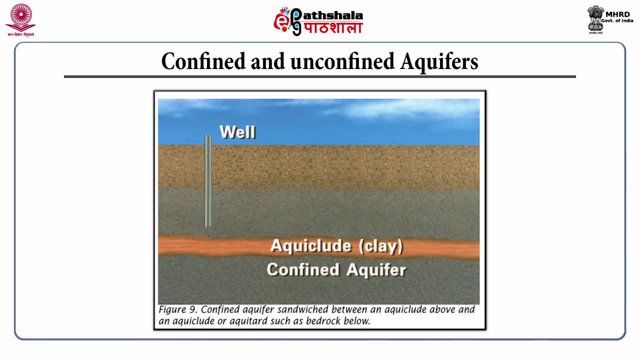 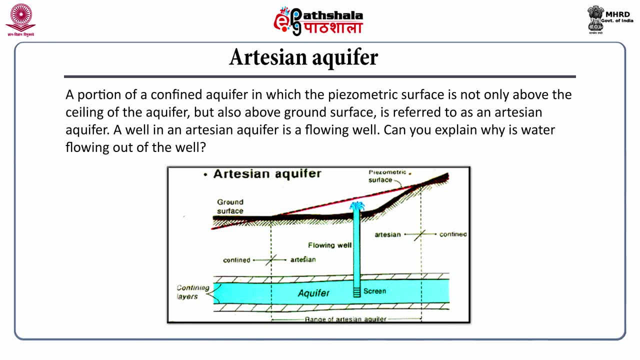 aqueclude here and the below to this aqueclude is the confined aquifer, Now artesian aquifer. artesian aquifer are the special case of a confined aquifer where the pressure in confined aquifer is so high that when we drill a well, hydraulic well 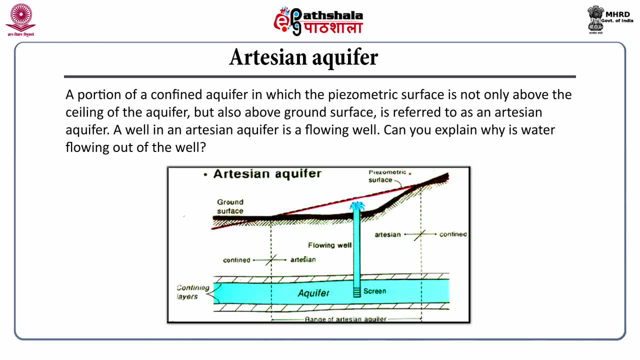 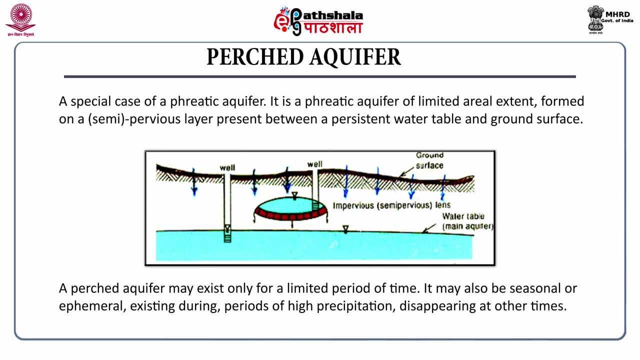 water starts coming out at the surface automatically without any pumping requirement. So these are known as artesian aquifers, where the water pressure becomes very high and there is no need of pumping of the water to bring the ground water sources at the surface. Passed aquifer is a special case of phreatic aquifer. It is a unconfined aquifer of very 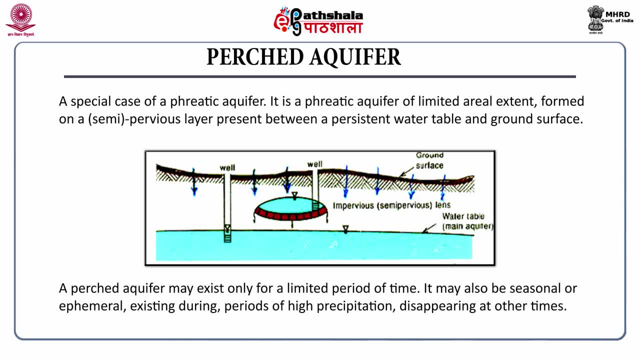 limited extent. This is formed over a semi-pervious layer that is present between a persistent water table and ground water surface. So ground water table is here and there is a ground surface. So in this unsaturated zone there is a semi-pervious barrier, very local. 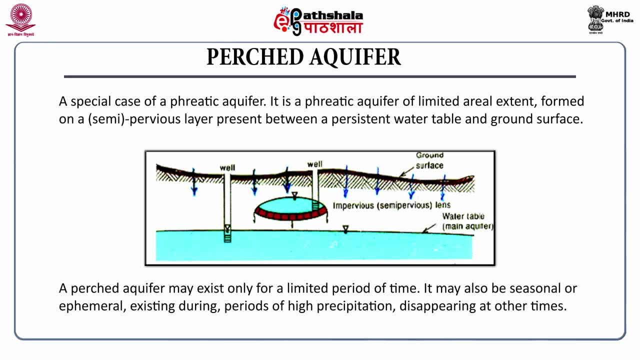 small formations. The water get stored during the monsoon season and when we drill a well, the water stored over this semi-pervious barrier depletes very fast. So such type of this aquifer are known as first type aquifer, mostly found in the dry region where generally we 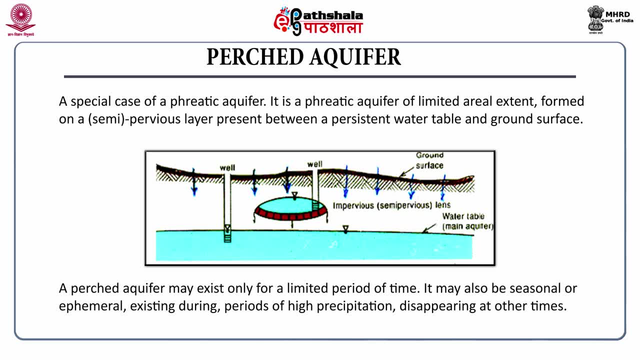 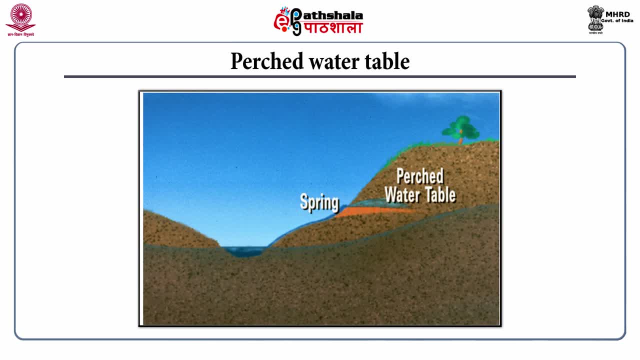 go from the plain region To the mountainous region and this is the example that how this first aquifer are going to be formed. the most of the springs which are generated in the highlands You can see a spring is the water is coming out or the surface from a spring and there is a small 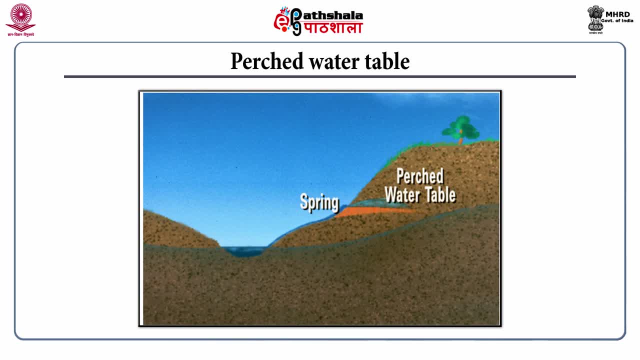 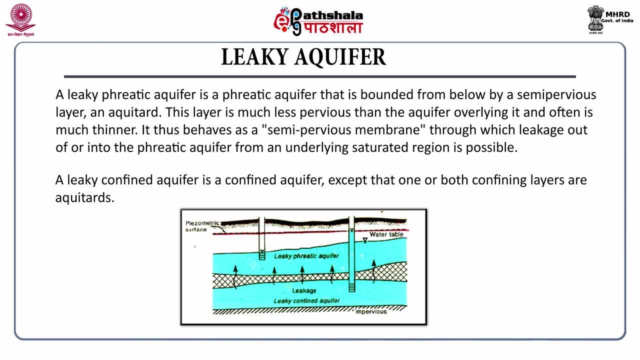 clay liner belonging to this first aquifer- Leaky aquifer- when this clay liner is going to be very thin. in that case transmission of the water in vertical direction may also be feasible. So such type of the aquifer which are having a very thin clay liner, which 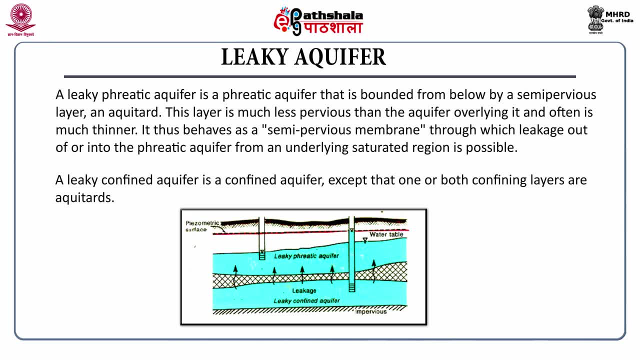 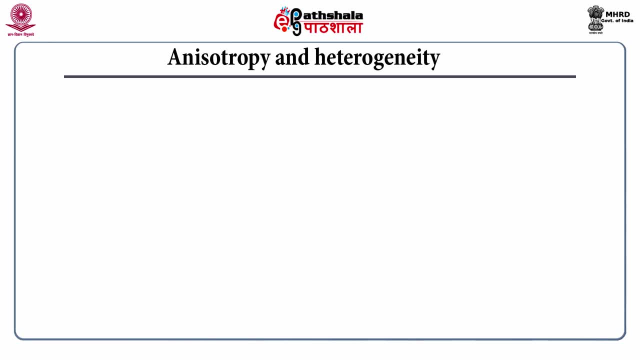 allows some sort of water interaction from in a vertical direction, or cold, as leaky, confined or leaky unconfined aquifer. Now to understand the groundwater, hydrology, anisotropy and heterogeneity is a very important parameters, especially most of the hydraulic models. we generally are based on the assumption. 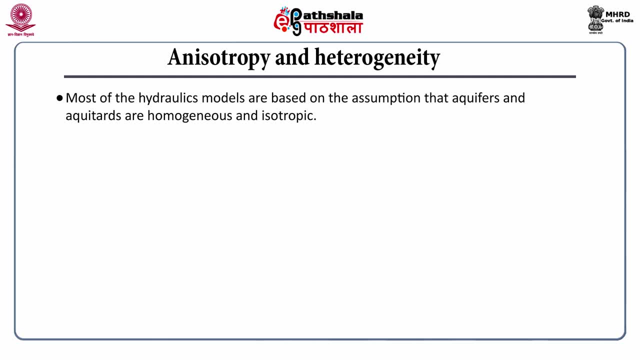 that aquifer and the aquitards are homogeneous and isoph trous, The two climbing thousand bisc psychologist, as I said, you know. And I think the first, isotropic Homogeneous means property of the aquifer material is same at everywhere and isotropic means in the properties are similar in each direction. This means that the hydraulic 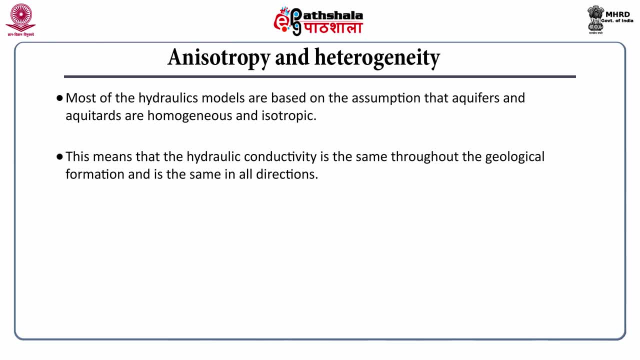 conductivity or other parameters are same throughout the geological formation and is the same in all directions. However, the particles of the geological formation are seldom in spherical nature. When they get deposited under the water, they tend to settle over a flat side. In such formation, hydraulic conductivity in horizontal or the 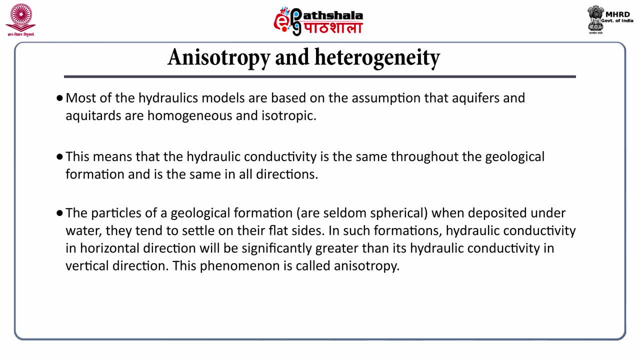 transfer direction are going to be much higher than the hydraulic conductivity in vertical direction and this phenomena is known as anisotropy. So flow of the water in horizontal and transfer direction is going to be much faster than the flow in vertical direction In horizontally. 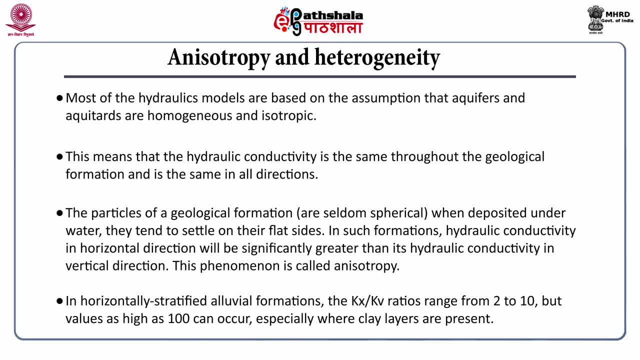 stratified alluvial formation. this ratio of hydraulic conductivity from k x to k y v is going to be between 2 to 10 times, and sometime it may be up to 100 times more. So it means water can flow 2 to 10 times fast in horizontal direction, as compared to. 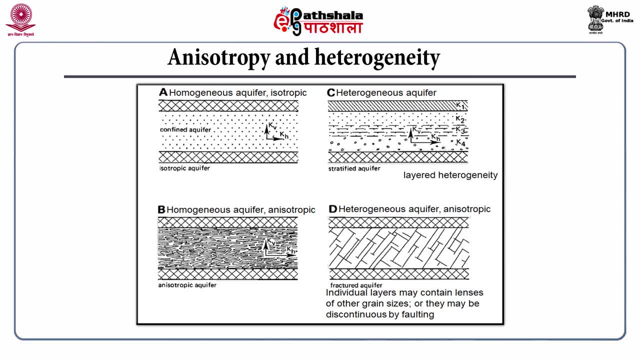 its vertical movement. This picture shows the distribution of the anisotropy and heterogeneity type of the aquifer material. You can see figure number a where the completely homogeneous and isotropic type of the media is there. So properties are same in at every place. 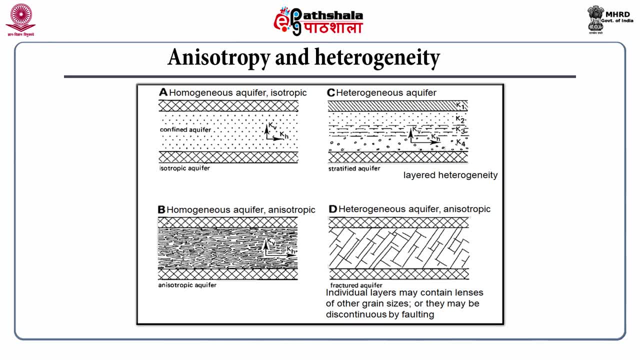 and also in each direction. Figure B shows that it is a homogeneous indeed, but the hydraulic parameters are different in x, y and g direction, So we cannot call it isotropic type of the media. So this is going to be homogeneous and anisotropic type of the aquifer. C shows the heterogeneous. 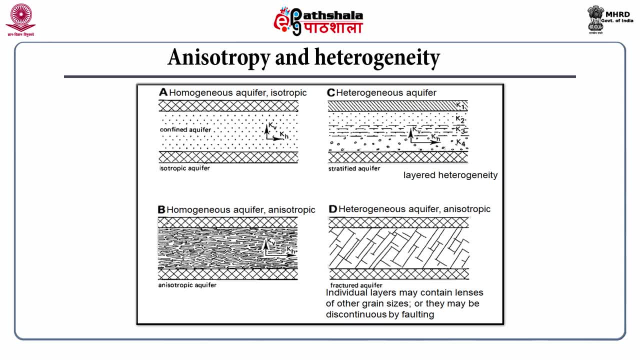 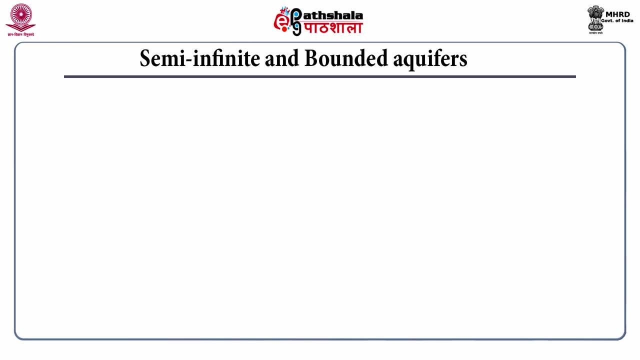 type of the aquifer where the different three layers are there and the last one is the heterogeneous and anisotropic having a fracture type of the media where the properties are different in different direction at an different places. The another important terms related to groundwater hydrology is semi-infinite and bounded aquifer. 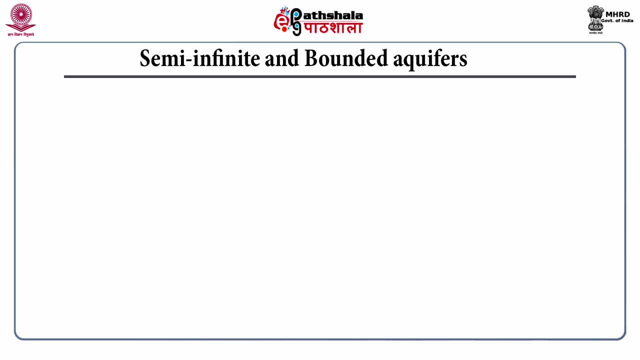 We see that this aquifer type is semi-infinite and it is a bounded aquifer. So a common assumption in groundwater hydraulics is that the aquifer is horizontal and of semi-infinite nature. that is means bounded in vertical direction and unbounded laterally. So it is aquifer's. 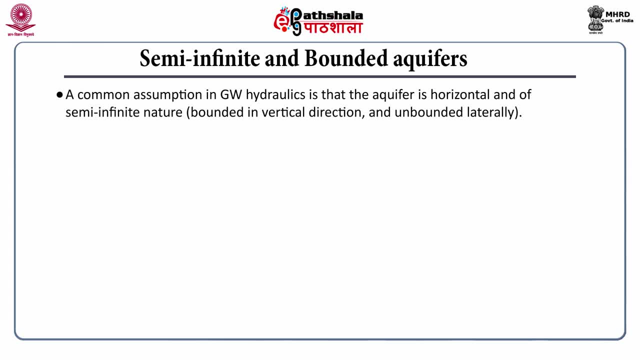 horizontal expansion is going to be much higher. Then it is vertical thickness. So vertical thickness is generally going to be may be up to 50 or let us say up to 100 meter, but it is horizontal and transverse extension going to be in kilometers and that is the region we call mostly aquifer as going to 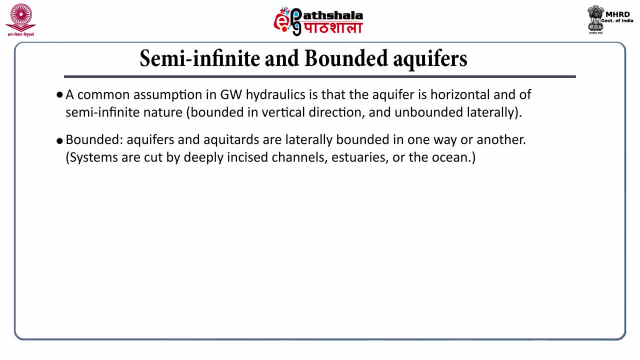 be of semi-infinite in nature. Bounded aquifers are also bounded vertically and these are the picture which shows the bounded aquifer where we can say vertical dike or a boundary improvised by, or may be, a river which is cutting through this aquifer. So the vertical boundary as well as the horizontal boundaries of the 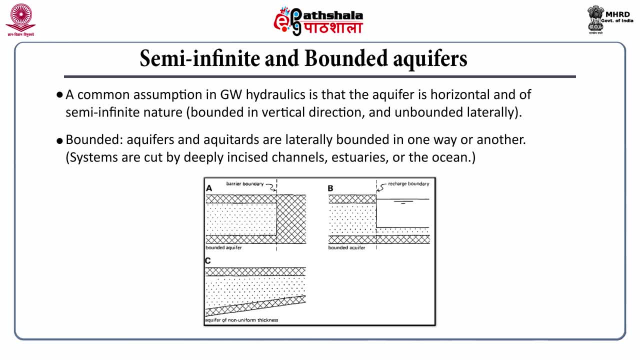 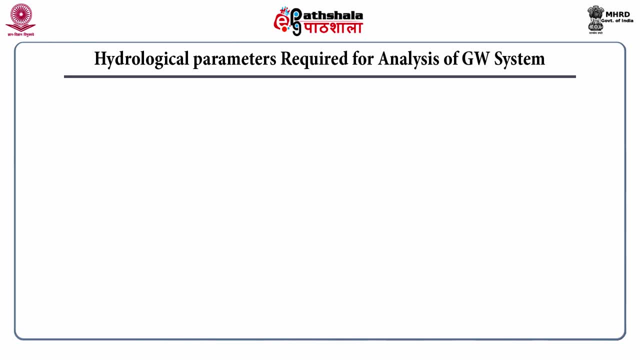 aquifers are bounded, and that is the reason we classify such type of the aquifers as bounded aquifers. Now, hydrogeological parameters are generally required for characterization of the groundwater sources. So these are the some parameters, like porosity, density, texture. 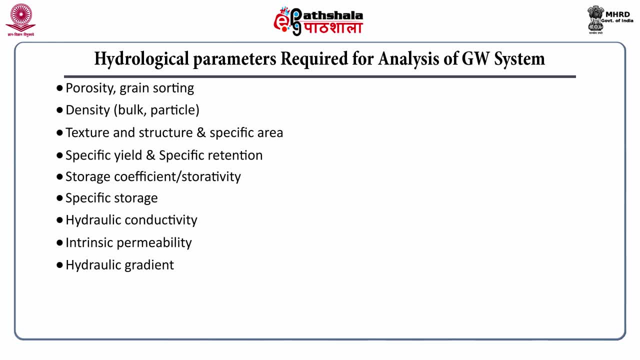 specific yield, specific storage, hydraulic conductivity, transmissivity and some other parameters which are related for the analysis of the groundwater hydraulics, which we are going to discuss one by one in the coming slides. The porosity of a rock is the property of. 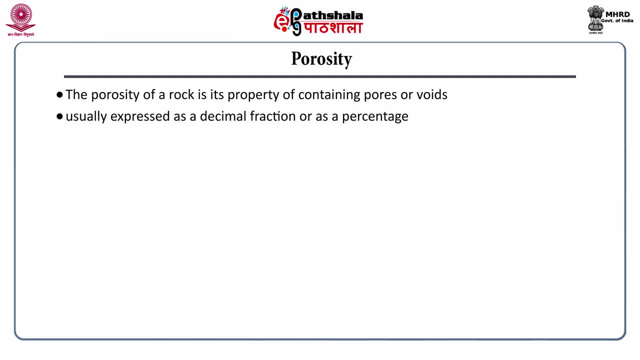 containing pores or the voids, usually expressed as a decimal fraction or as a percentage. We can classify porosity either as absolute or effective porosity and are distinguished by their excess capability to groundwater. So total or the absolute porosity is the total void space. 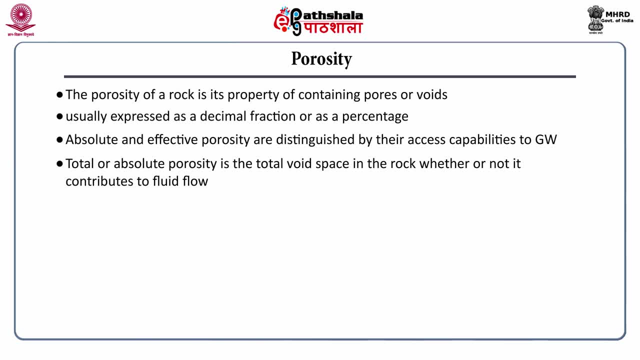 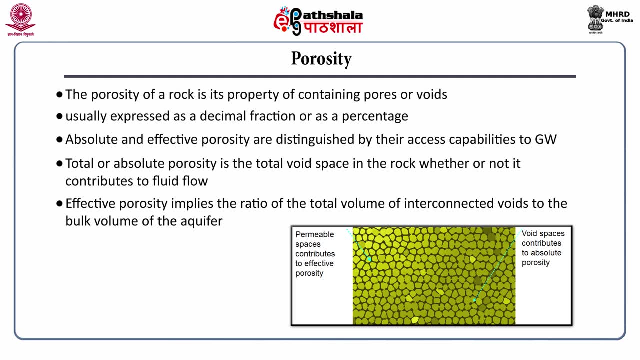 in the rocks, whether or not they are porous. So the porosity of the rock is the property of, not it contributes to flow of water. Effective porosity implies that ratio of the total volume to interconnected voids only. So in this picture you can see most of the openings. voids are connected. 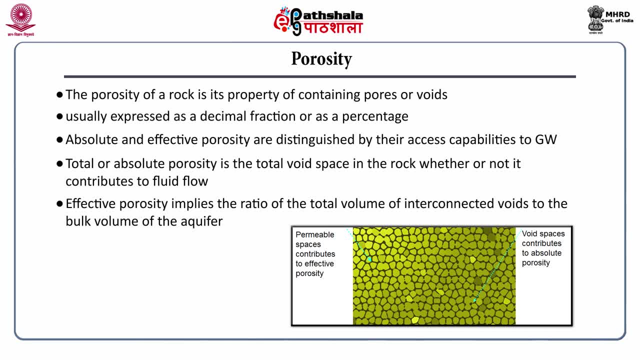 and they can contribute to the groundwater flow. But there are some minute voids which are completely disconnected from the rest of the soil mass, rest of the surrounding voids they cannot contribute to in the groundwater flow. So if you exclude such type of the openings from the total, 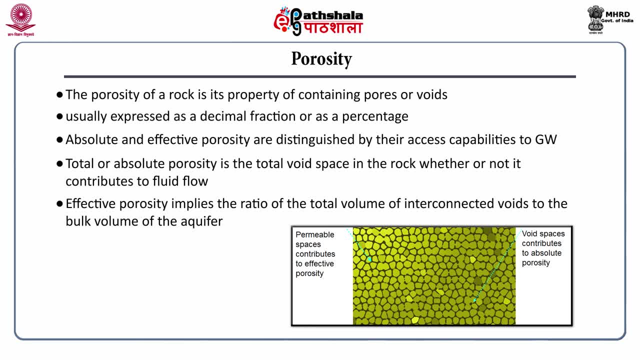 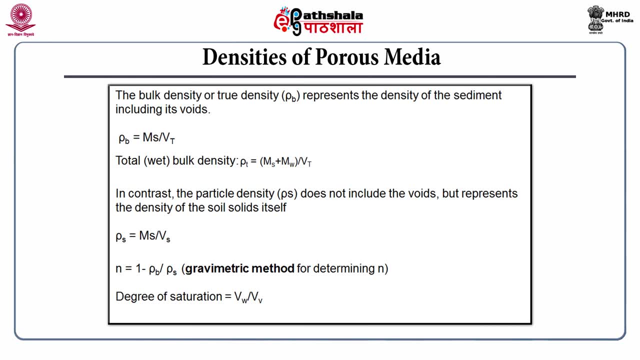 porosity, we get the effective porosity. So the porosity of the rock is the property of the effective porosity which is going to contribute in really for the flow of the groundwater in aquifers. Densities of the porous media, the bulk density or the true density. generally we classify the bulk. 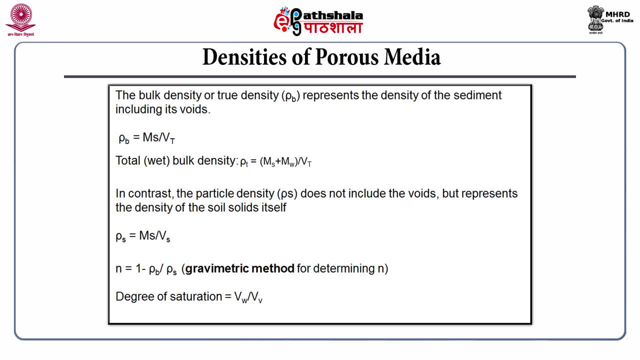 density by considering the entire volume of the aquifer material, The particle density generally. we consider only the volume of the soil, solids, geological materials. So particle density is going to be higher than the bulk density and we can get the relationship between the particle and the bulk density with porosity of the geological media. So porosity, an is. 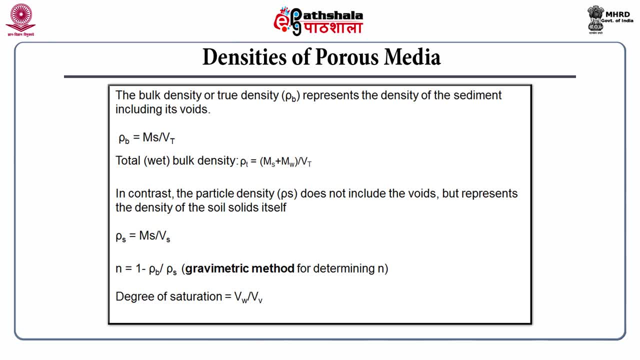 going to be equal to 1 minus rho b, that is the bulk density divided by the rho s, that is the particle density. Sometimes we also represent degree of saturation of the geological material, especially for the w ê d o d zone and saturated zone, where it is the ratio. 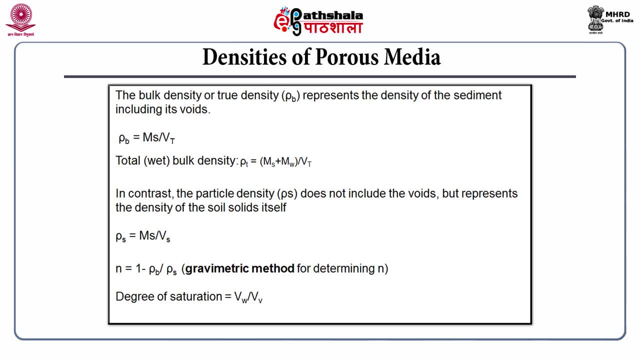 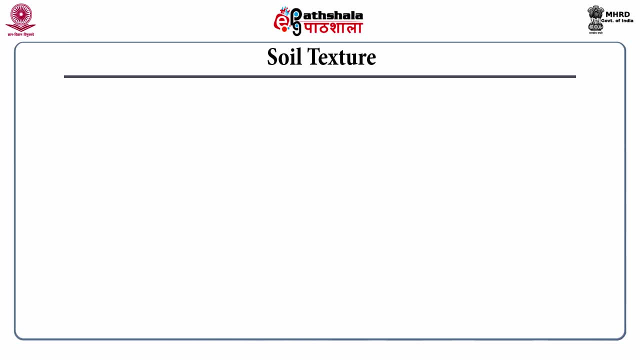 of the volume of water to the total volume of the aquifer material. Soil structure and texture are generally for this unsaturated zone. texture means that how the soil particles are arranged with each other, and soil texture means the size of the soil particle by which this aquifer material is made of. 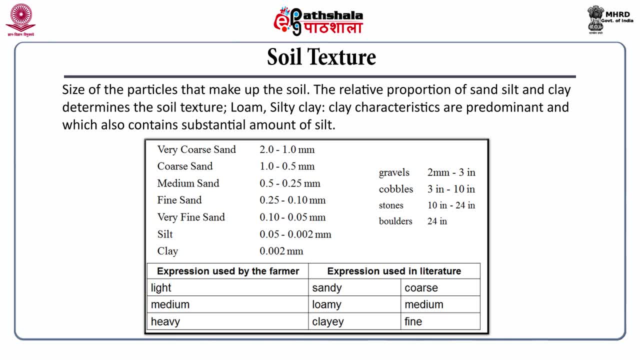 Soil texture can be classified based on the size of the particle, like very coarse sand, medium sand, fine sand, silt and clay, and mostly it is used for the soil classification triangle provided by USGS. Specific area is the area per unit weight of the aquifer material, especially for the 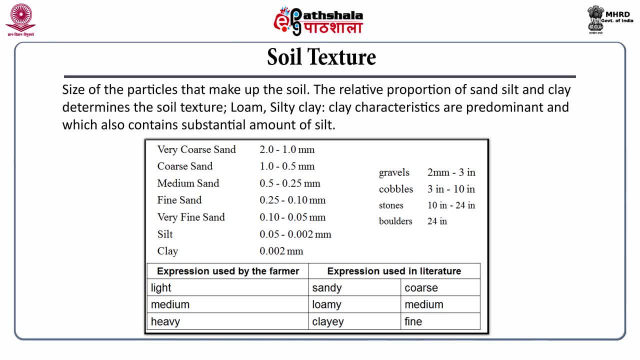 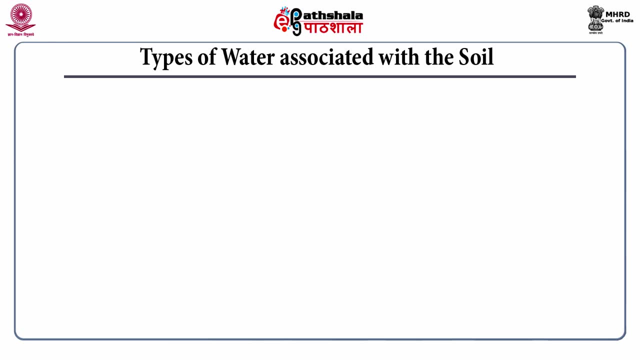 groundwater quality point of view specific area plays very significant role in the improvement of the water quality. smaller the particle size of the aquifer material, more is the specific area. Now question comes that how this groundwater is stored into the porous media. so this picture. 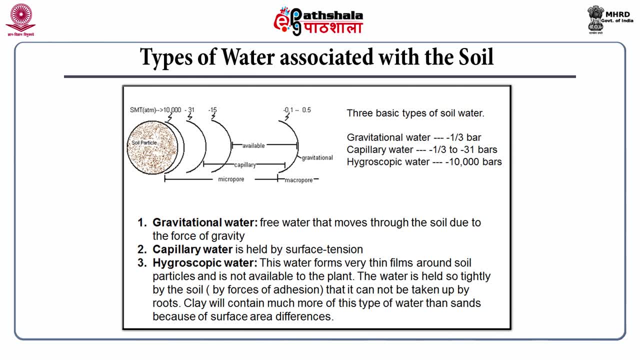 shows that soil particles, Soil surface is there? any geological particle is there? surrounding to this geological particle, there is a first layer of the water which is bounded because of the hygroscopic water. that is the pressure, though the force attraction between the soil particle and the water molecules. 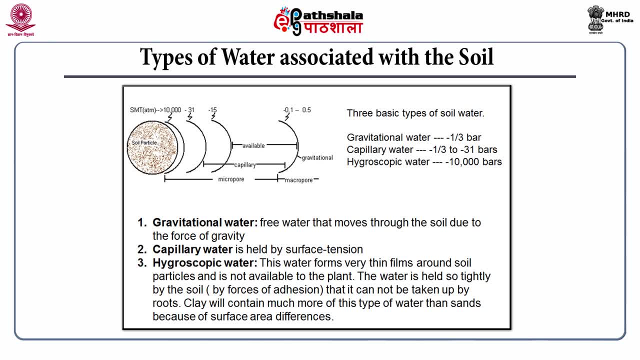 and then there is a capillary water and the last one is the gravitational water. So if you will take a saturated geological material and if you allow this saturated material to drain because of the gravitational force, The water started, you know, dripping from the saturated soil mass and that is the gravitational. 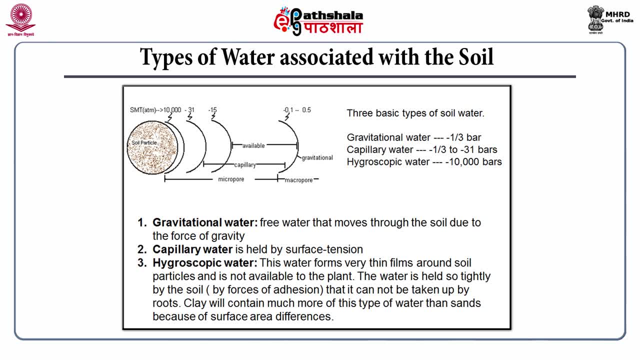 water. So gravitational water is the free water that moves from the saturated soil due to force of gravity, and the remaining water into the soil or aquifer material is going to be capillary water and the hygroscopic water. Hygroscopic water is so tightly held that one cannot extract this water under ordinary. 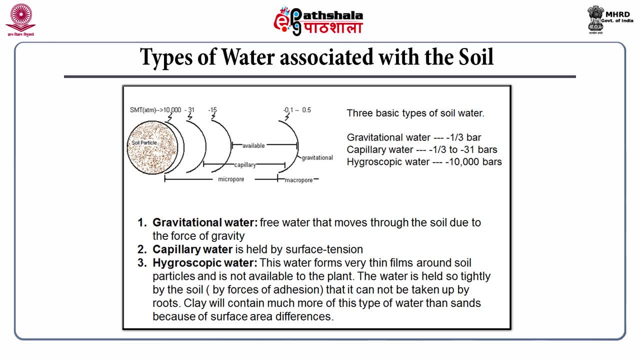 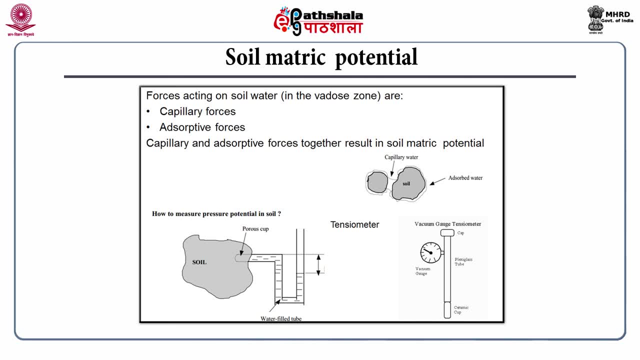 conditions, even in weather zone, plant cannot extract this hygroscopic water from the weather and the humidity, whereas from the soil mass, Soil metric potential and the soil moisture content are the these two units which are used for measurement of the water content in unsaturated zone. 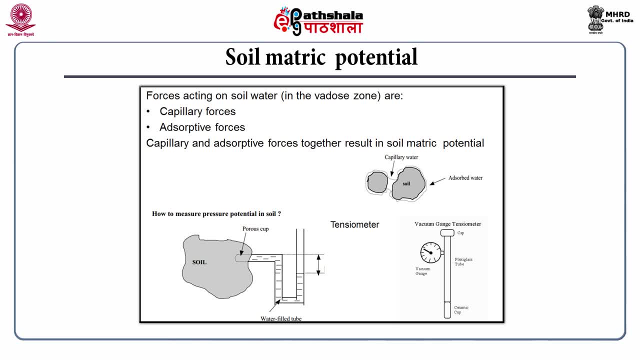 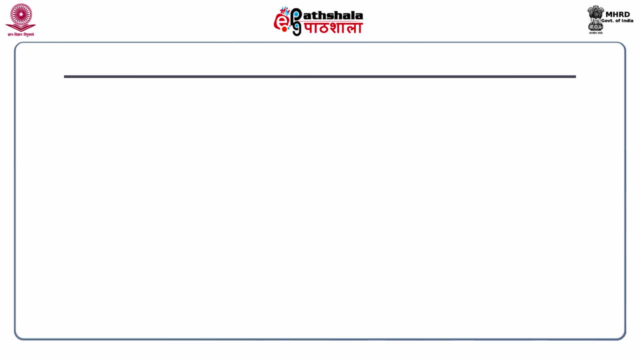 Soil metric potential is the head of the water column generally. it is going to be section head for unsaturated zone and it is going to be 0 for the unsaturated soil. Soil moisture content is represented by theta. this is the volume of water divided by the. 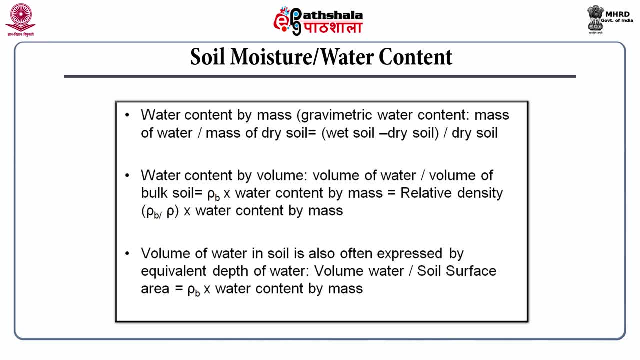 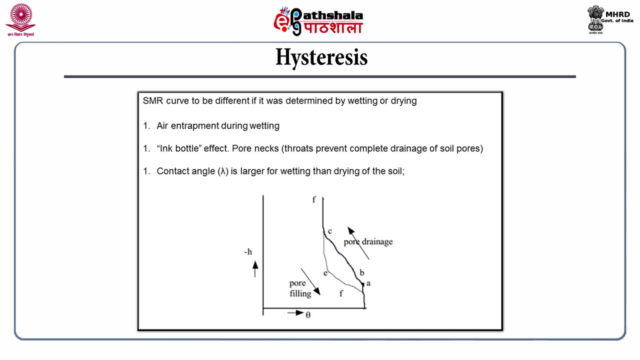 total volume of the soil mass. So that means soil mass or the aquifer material. So this is going to be a unit less type of the parameter which is mostly used for the quantification or analysis of the unsaturated hydrology Hysteresis when we drain or when we fill the pores of the soil particles. the relationship: 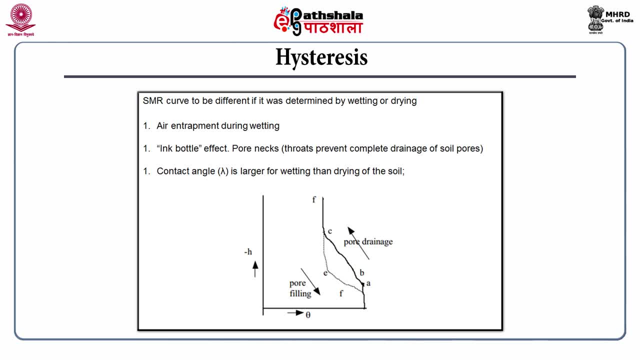 between the soil metric potential H and the theta are not going to be akin, they are going to be different, and the this difference is known. this process is known as hysteresis. Now for aquifer specifically, we are having two important parameters for unconfined aquifer: the 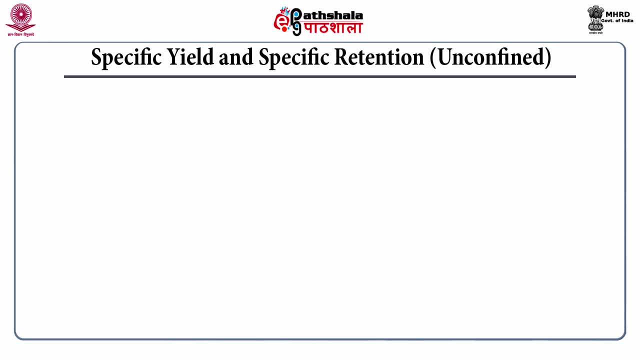 first one is the specific yield and the second one is the specific retention. Specific yield is denoted by Sy and specific retention is denoted by Sr, So which, whatever the water which is stored in the pores, cannot be drained by the gravity by the pumping. So the volume of the water 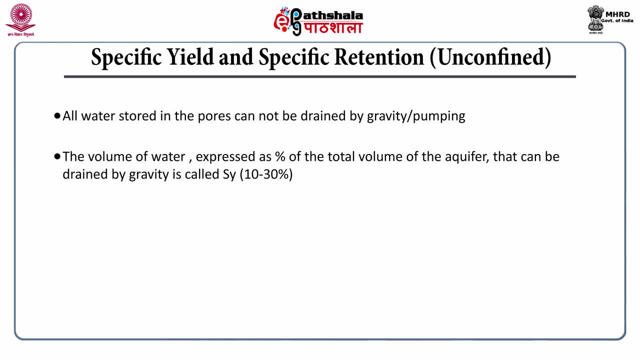 which is expressed as a percentage of the total volume of the aquifer which can be drained by the gravity, is called as specific yield, and the volume of the water that is retained by the porous media against this gravity force is known as specific retention. again, it is represented in percentage. 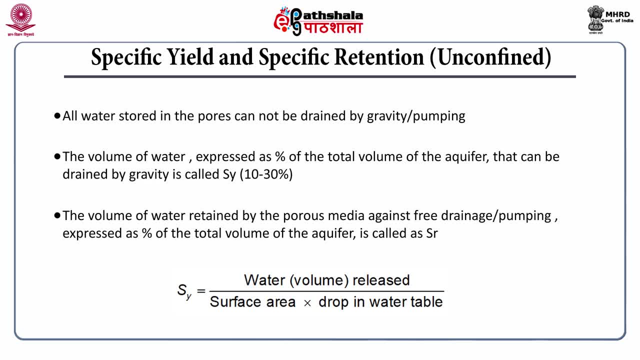 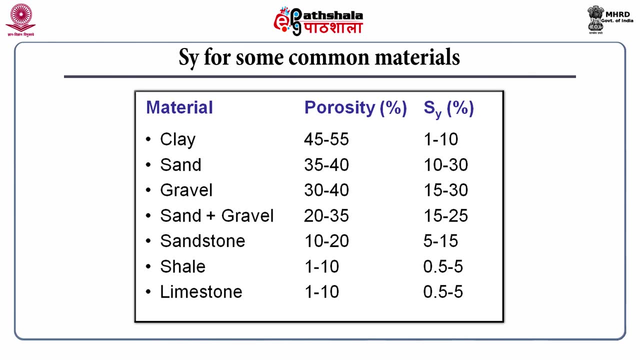 So a specific yield is the volume of water released per unit volume of the aquifer material and if we take this from the total porosity we are going to get the specific retention. These are the some typical values of the specific yield for different type of the geological material comprising this aquifer, For example clay. the porosity: 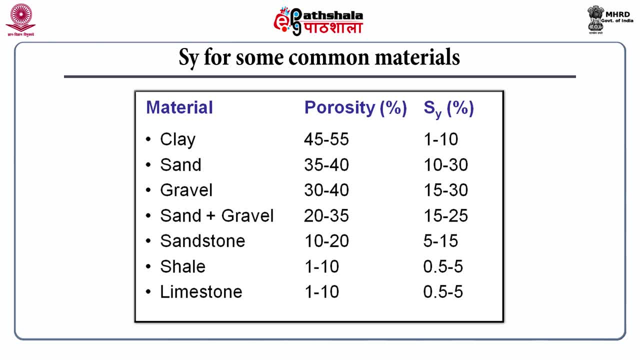 of the clay is high, but its specific yield is very small: 1 to 10 percent, only Sand or the gravel mix. its porosity is not so great as compared to clay, but specific yield is very high, varying from, let us say, 15 to 25 percent, and that is the reason that we denote that. 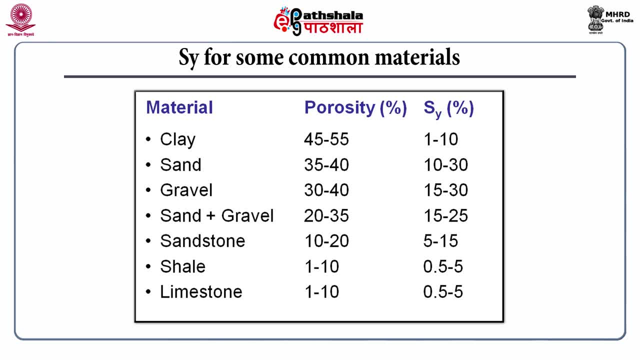 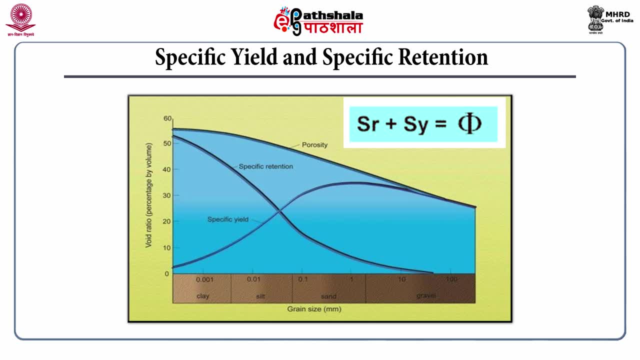 sand and the gravel mix are going to make the good aquifer material. This figure shows the relationship between porosity, where it is represented by phi, a specific yield, Sy and specific retention. If you look at this diagram, the y axis shows the void ratio and the x axis shows the grain size which is increasing in the x direction: 0 to. let us say some. 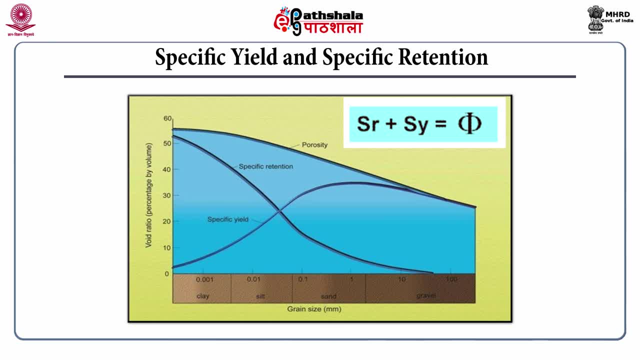 value when we go towards the x direction. So the top line shows the porosity, Top solid line. so initially when the size particles of this soil material is very small, for example clay, the porosity is very high. and when you go towards the increased grain size, the porosity. 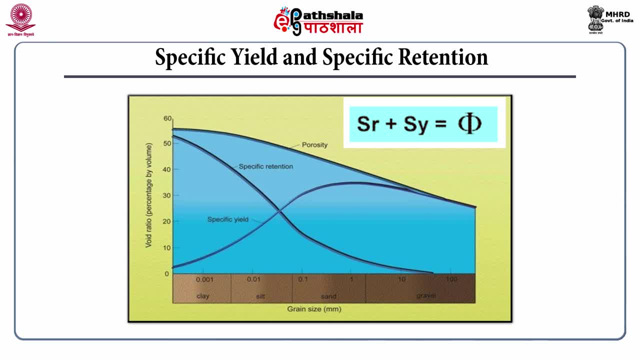 started decreasing Now. the another diagram, which shows the specific retention for clay, is very high. it is started, you know, decreasing when you go towards the sand or any coarse material. In opposite to that, the specific yield is going to be very small for clay, but it is. 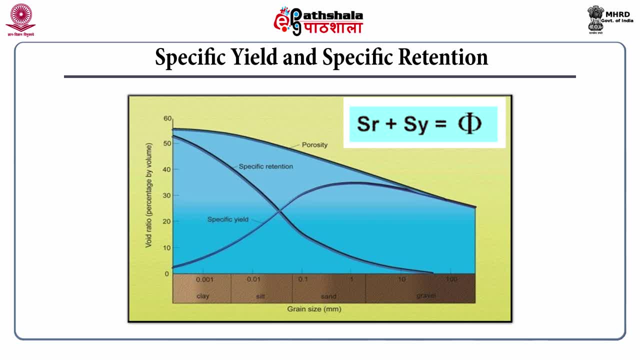 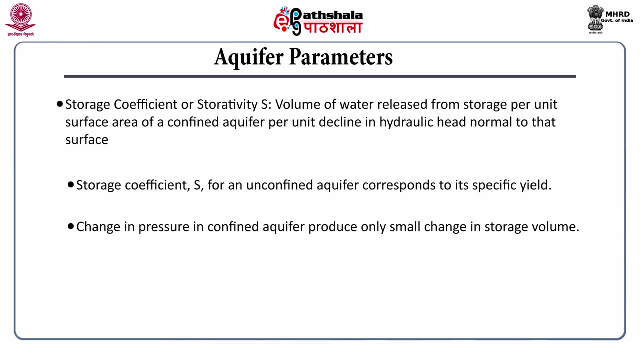 very significant, very high for coarse material like sand or the gravels, And the summation of this specific yield and specific retention are going to give the total porosity phi. Similarly for the confined aquifer we can say. for the other aquifers we can say storage. 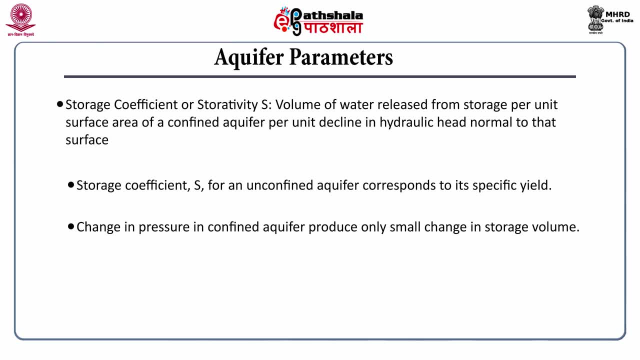 coefficient that is also known as storativity, denoted by capital S. So volume of water which is released from the storage per unit surface area of a confined aquifer per unit decline in hydraulic head normal to that surface is known as the storativity or storage coefficient. 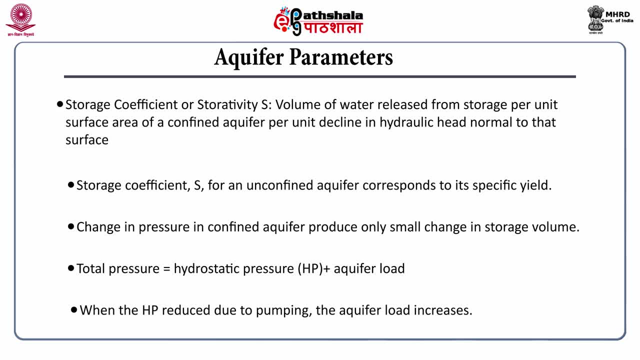 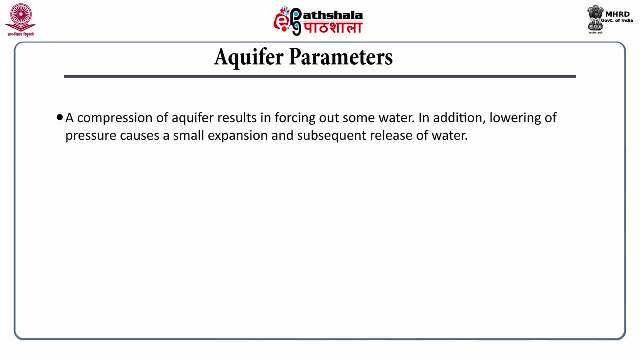 The total pressure in confined aquifer is going to be hydrostatic pressure plus the aquifer load, And a compression of the aquifer results in the storage coefficient, So difference in the forcing out of the some water. in addition, lowering of the pressure causes a small expansion and subsequent release of the water, So water released by the compaction. 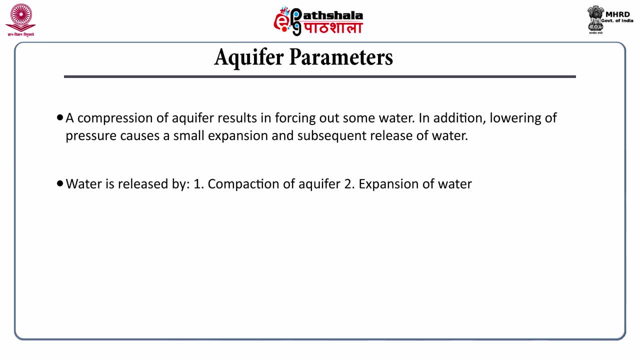 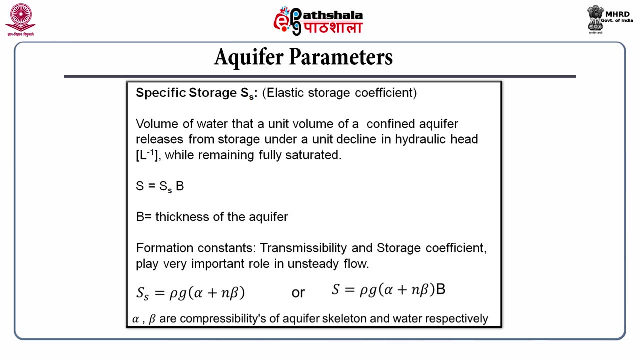 of the aquifer as well as the expansion of the water. So value of typical S value is going to be very small, 0.005 to 5, into 10, to the power minus 5, but for the water table aquifer the specific yield is going to be 10 to 30 percent. Other parameters for aquifers: 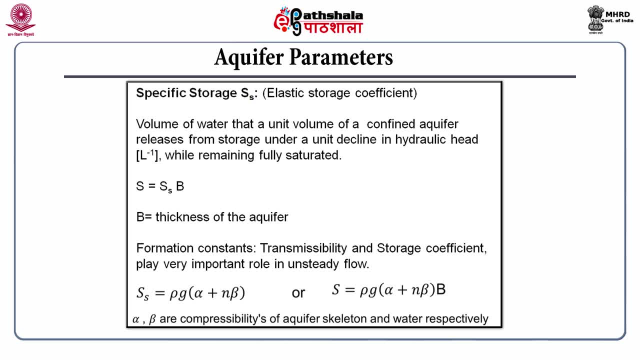 is also known as specific storage coefficient. So water in confined aquifer is going to be 10 to 50 percent, and with the water being s s. So if you divide this storage coefficient s with the total thickness of the aquifer, we get the specific storage, And specific storage and storage coefficient can be denoted. 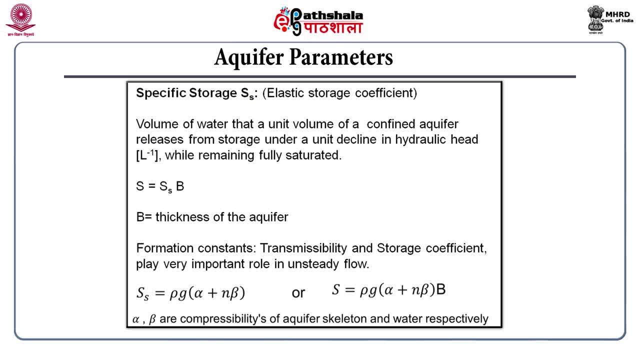 by this compressibility of the aquifer, kilton, and the water compressibility. this s is going to be rho g, alpha plus neta, that is the porosity into beta, into B capital. B is the thickness of the aquifer And alpha and beta are the compressibility of aquifer and the water respectively. 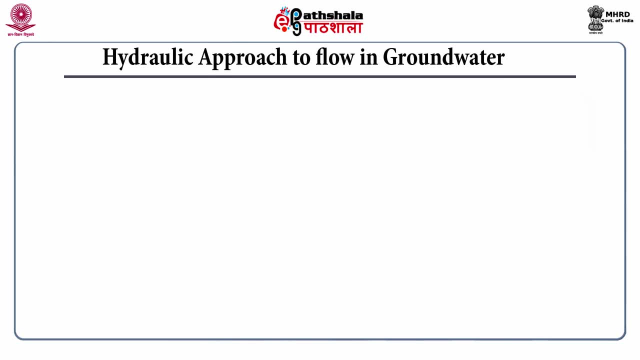 Now for hydraulic approach of the flow in groundwater. we generally go from 3-dimension to 2-dimension. generally because most of this exception, like hydraulic well or the coastal region and root water, uptake where the flow is going to be in 3-dimension. otherwise we 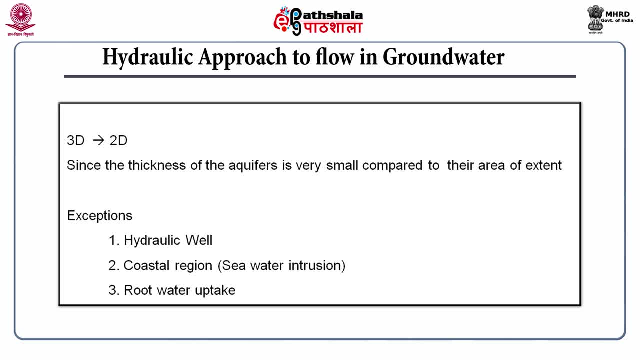 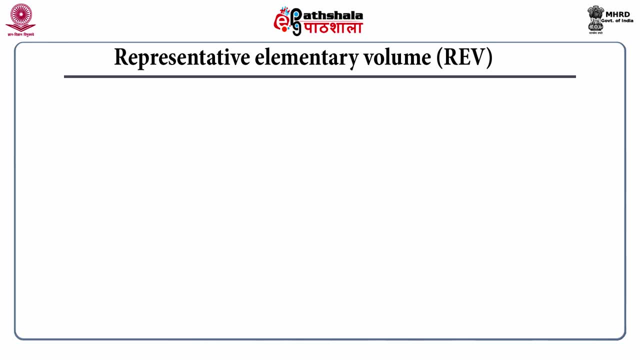 can represent the groundwater flow in a 2-dimension with some accuracy. Now question come that: at what scale somebody should analyze the ground water flow? So whether it is going to be field scale, large scale, very small scale, pore scale, So the 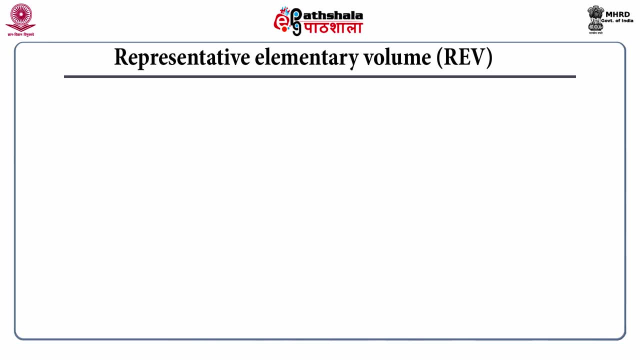 term which is used for most of this models which are representing groundwater. you know, flow and contaminant transportation are at REV scale. So REV is nothing but representative elementary volume. So REV is the smallest volume over which a measurement can be made. that will be value representative of the entire, of representing the entire aquifer Below. 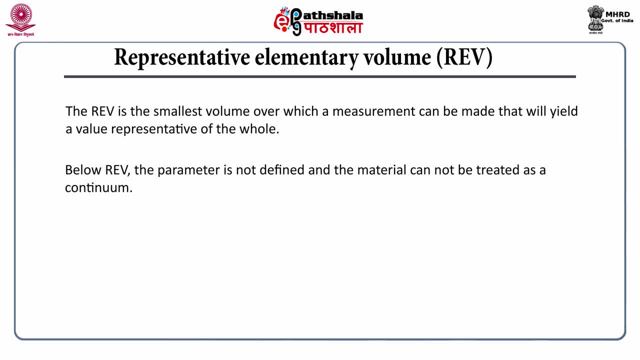 the REV, the parameters not shown. So REV is not defined and the material cannot be treated as a continuum. and if the sample of the aquifer becomes very small, the reading tends to oscillates. We are not going to get a consistent reading of the aquifer parameters. As we increase the sample size, the oscillation. 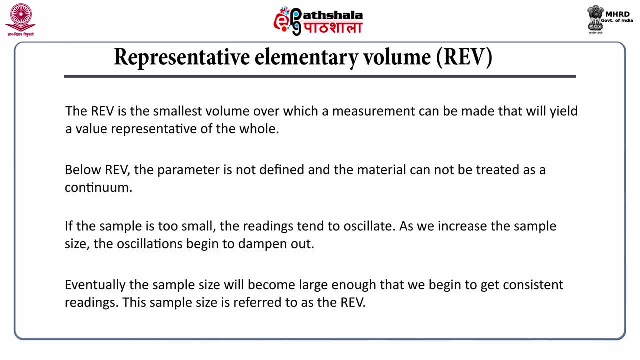 begins to dampen out and eventually we get a sample size which is large enough and we are going to get a very consistent value of the aquifer parameters. So that volume, where we get the consistent value of the aquifer parameters, is known as REV. So REV is not. 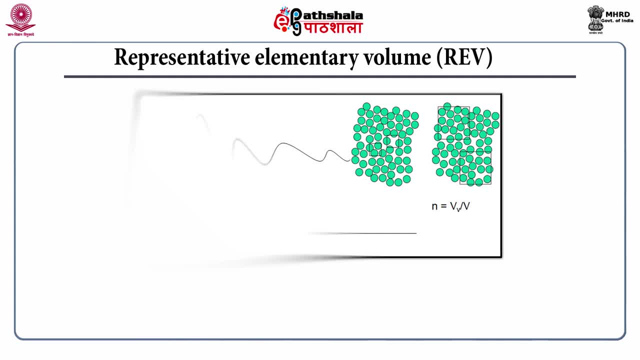 defined as a representative elementary volume. This picture shows this REV concept more clearly. You can see here there are two soil samples on the right hand side, The first: we take a very small soil sample. Now, by considering this soil sample, small soil sample, one sample. 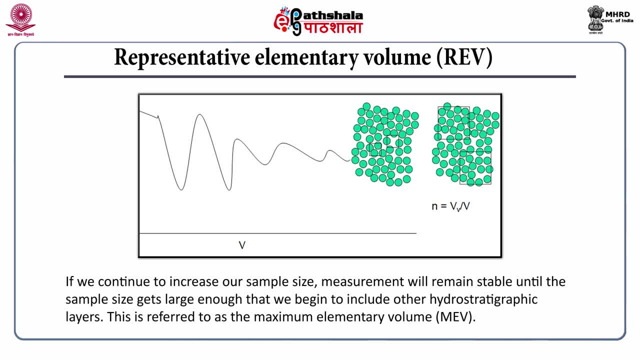 is having more voids as compared to the another samples, which is having more soil solids. It means the porosity is going to be very, quite differently for the same sample size. So but if we will increase the sample size that is denoted in the right hand side picture. 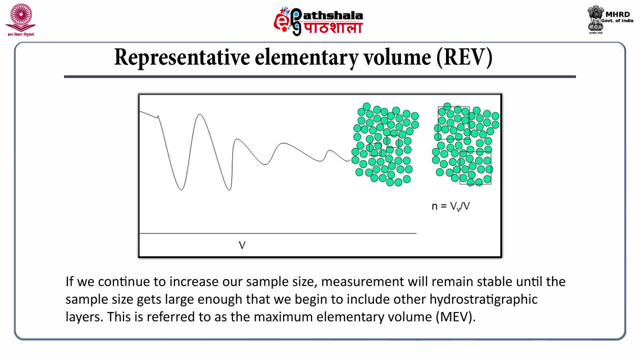 In that case, relatively, the difference in N is going to be low, and that is represented in this graph also. So the porosity oscillates very significantly when the sample size is very small. When we increase the sample size, this oscillations becomes now damping out. 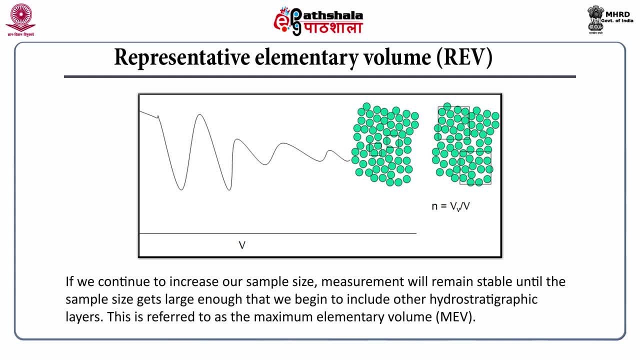 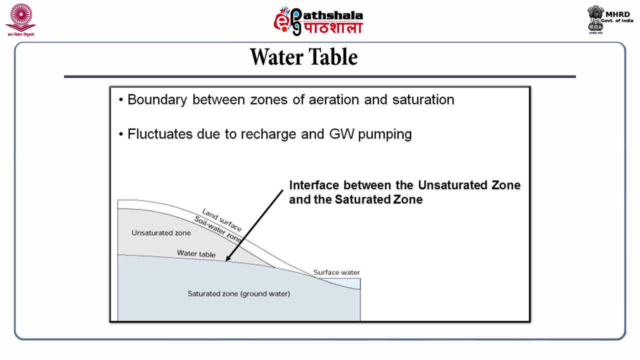 and finally we get a consistent value. that is the REV. Now, water table is a boundary that bifurcate this unsaturated and the saturated zone And ground water table is. if you look at the more closely, and nearby to the ground water table there is a capillary fringe where most of the soil particles, let us say up to few centimeter. 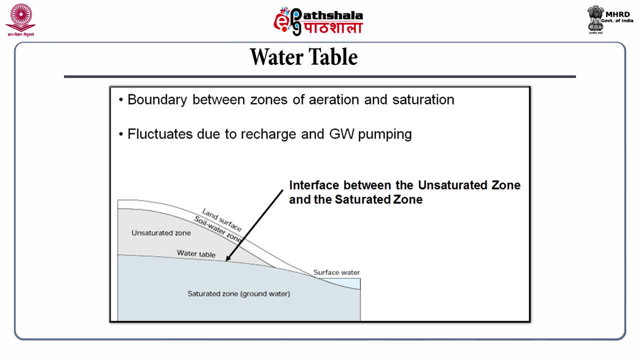 depth are going to be fully saturated. So because of the capillarity action, capillary action and the surface tension, the some portion of the soil mass is saturated. that is known as capillary fringe, And capillary fringe is somewhere lying above the water table which divides the weather. 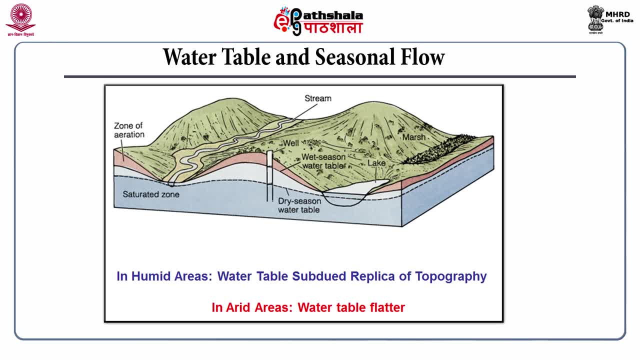 zone and the saturated zone. Water table is a not a constant phenomena. water table is going to be, you know, going to follow the surface topography during this wet season. Wet season means when there is a some flux from the top of the surface. then we can say the shape of 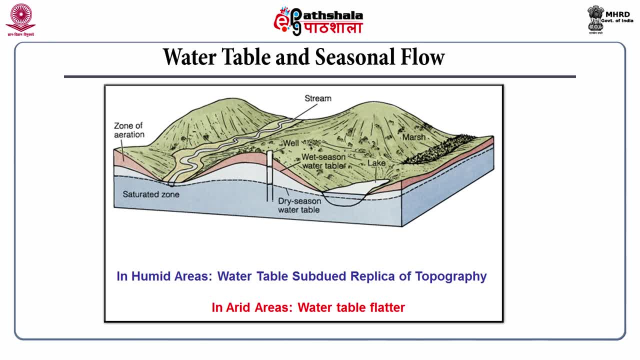 the ground water table is going to mimic the surface topography, But during the dry season, when this is a no flux recharging flux from the top, the ground water table try to, you know, become a plane, straight plane. So instead of following the surface topography, ground water table is going to be more flatter. 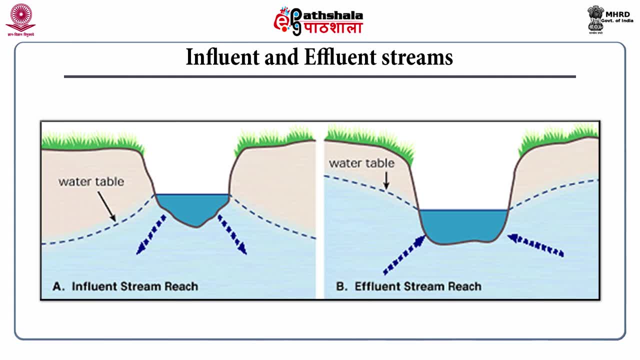 in dry conditions. Indeed, surface and ground water are not interrelated. you know separate entities. Both these resources are inter connected well with each other. in this slide you see there are two pictures, one on the left hand side and another on the right hand side. 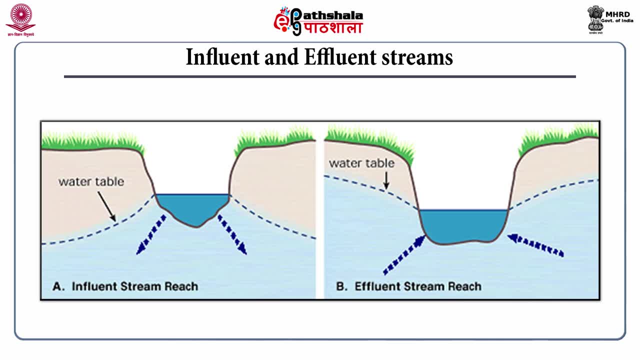 In the first picture the water table in the stream is above to the ground water table. It means water is going to enter from the stream to the surrounding soil mass and that is the reason we call such type of the streams as a influent streams. 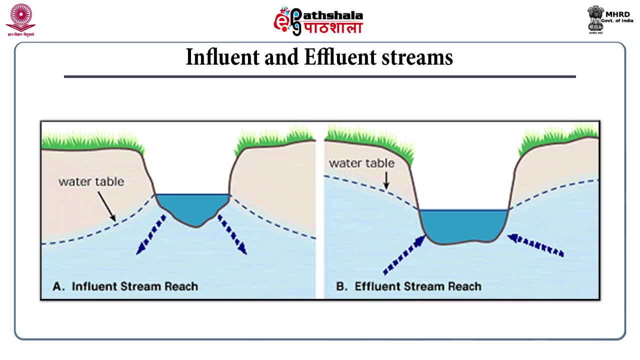 So these are the water contributing stream to the ground water. In second picture where the ground water table is more, you know, higher, you can say above to the surface water table in the stream. In that case ground water is going to contribute to the stream and such type of the stream. 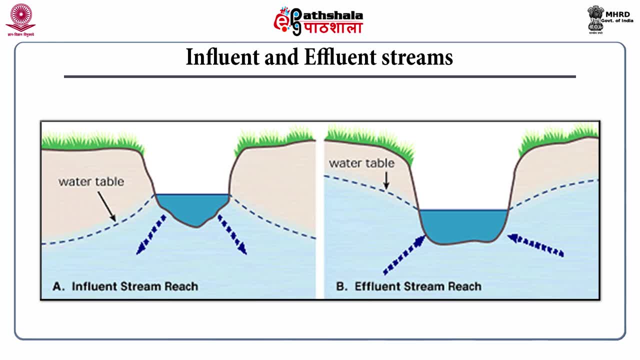 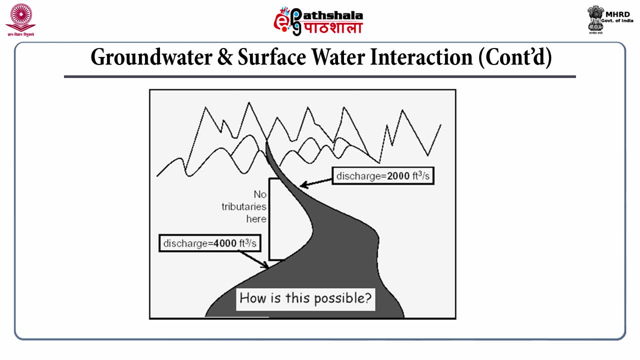 are known as affluent stream or gaining streams. This is the picture which shows a stream which is originating from a highland and then it is entering to the plane. There are two cross sections. cross section 1: the total discharge is 2000 cubic feet per. 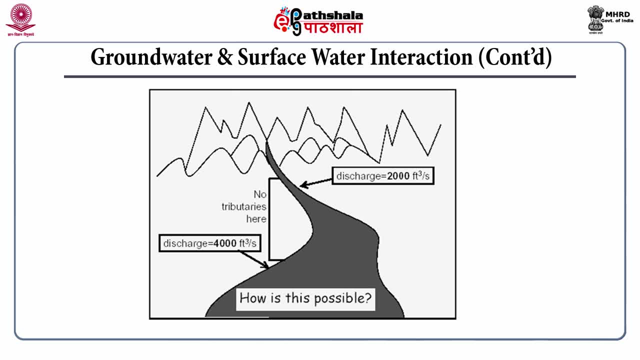 second and at some other down gradient side, the discharge is twofold, That is, 4000 cubic feet per second. There is no surface stream which is meeting between these two section. However, the discharge is increasing here. The reason behind that that the base flow that is contributing from the ground water.